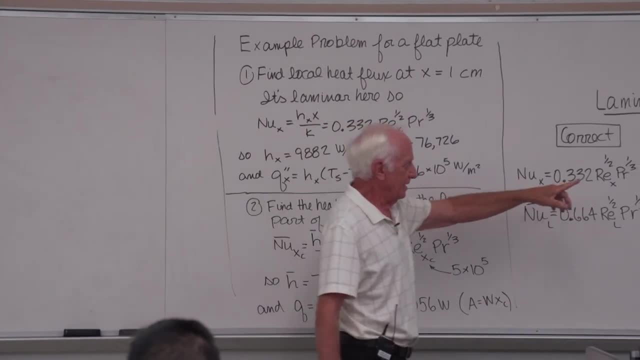 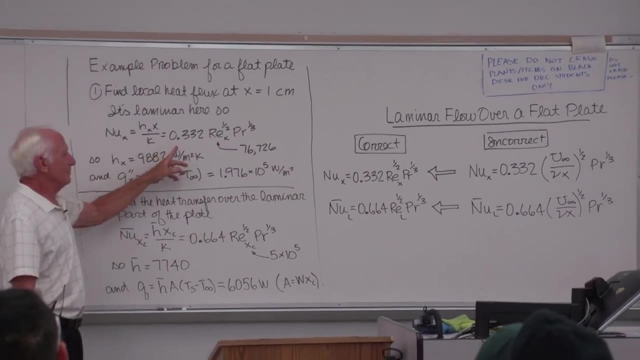 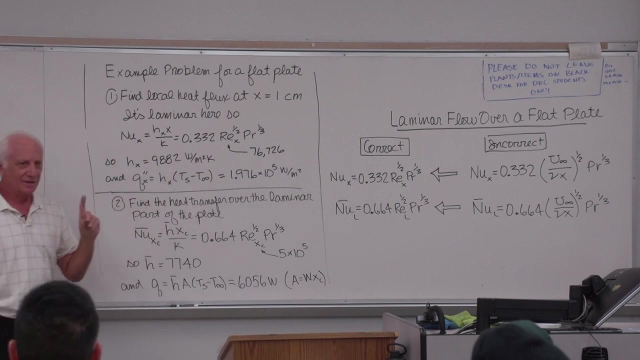 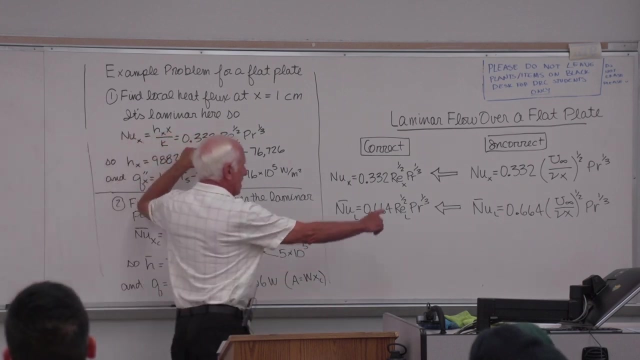 equation that's in your notes. is this one which is incorrect? It should be this one there. I used the correct one in my numerical calculations, So the answers are all numerically correct. It's just I copied the wrong equation down from my notes to the board, So this is the equation you. 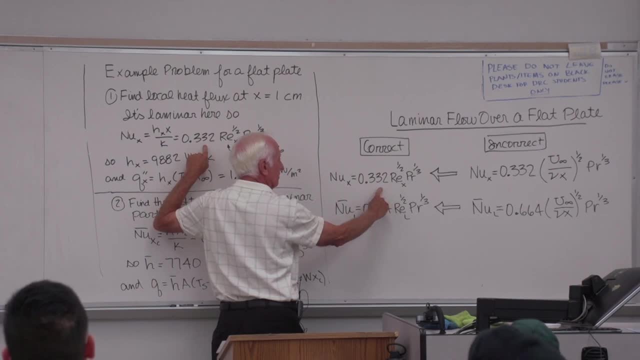 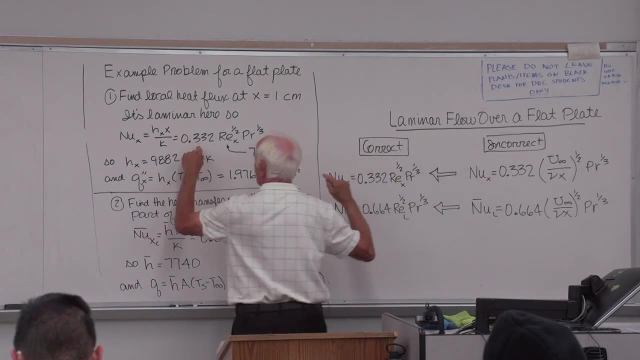 want to replace in part one of the example problem. Cross him out. This is the one that appears in here on the board that day. Cross that guy out in your notes here and replace it with the correct one right here. 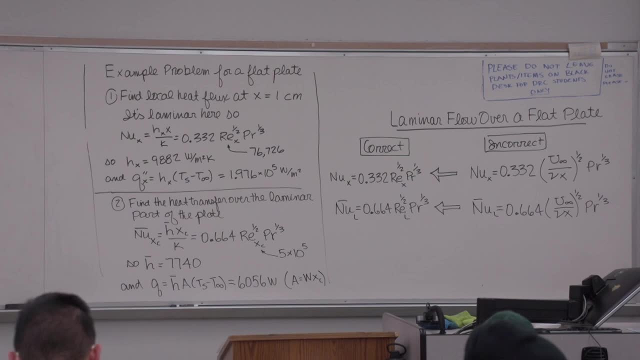 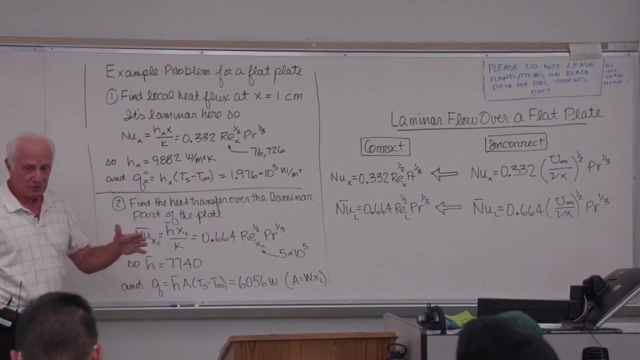 laminar part of the plate. Okay, So it's laminar, but now you want the bar because it's over a certain region. So now, this is the correct equation. The one in your notes is probably this one, right here: 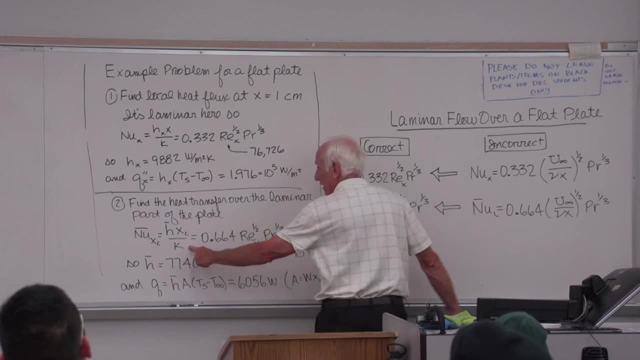 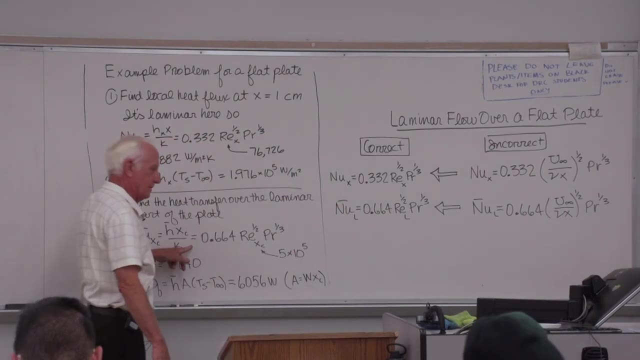 which is incorrect. So cross that guy out in Part 2 on that line and replace it with the correct one, which is right here. But again, the numerical answers are correct because I just copied the incorrect equation from my notes to the board. 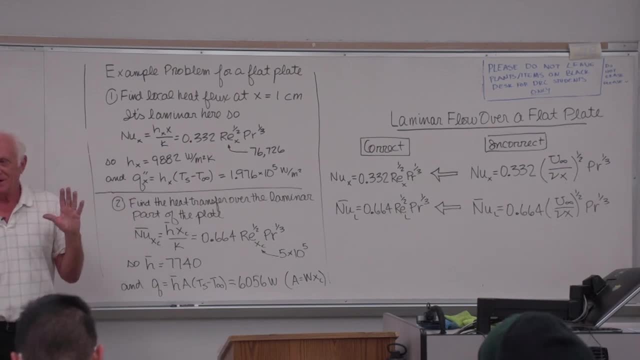 Okay. So just so you get the right equations on your equation sheets for the third midterm. you don't want the wrong equations on your equation sheet, So the correct ones are on the board over there now. Okay, Any questions on that? Okay, Just a reminder. Chapter 6,. 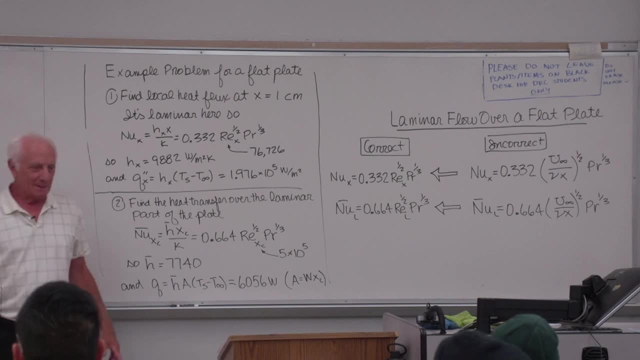 7 homework due today. the third midterm will cover Chapter 6,, 7, and 8, and we'll talk more about that on Friday and Monday, But the third midterm is a week from today. a week from today, next Wednesday. 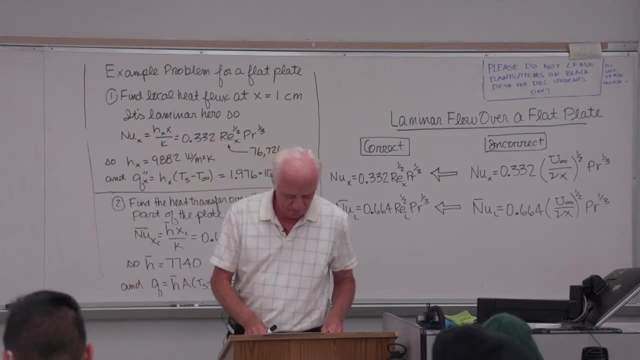 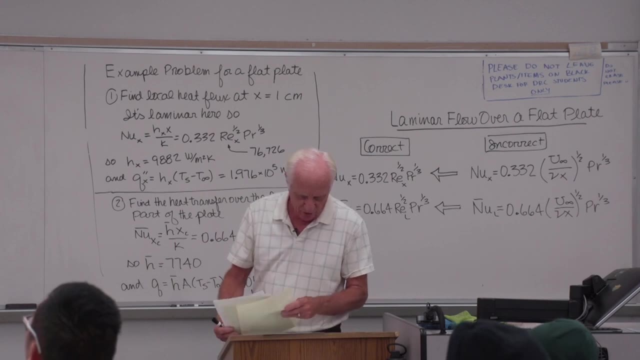 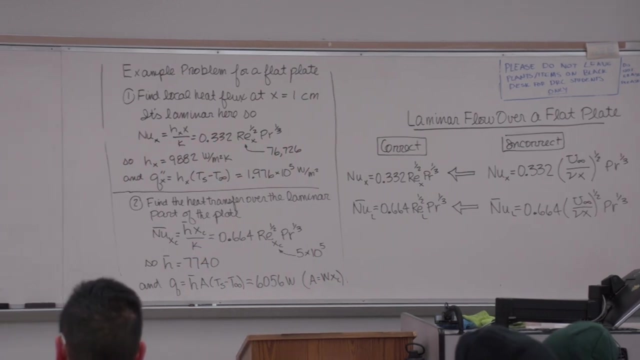 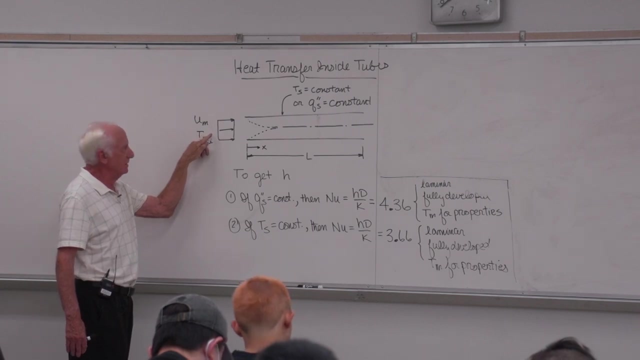 Okay, So go back now, return to Chapter 8, and we're looking at flow. Here we have a flow in a tube and so the flow in a tube picture over. here we have a uniform velocity profile, the velocity's u subscript. 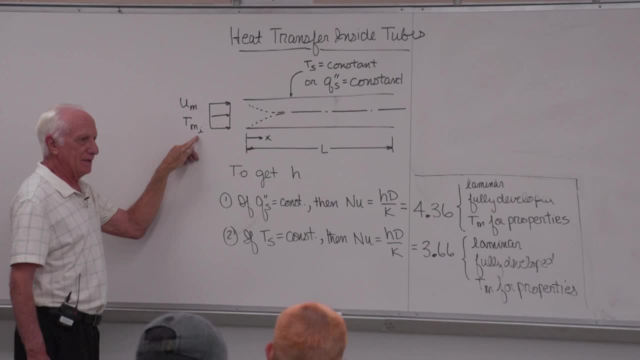 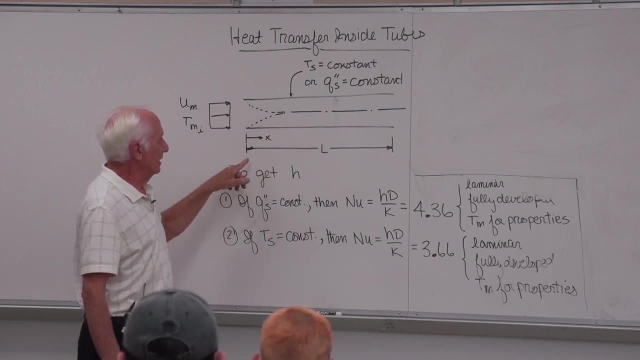 means the mean velocity entering the tube. We have the mean fluid temperature at the inlet T, mean i uniform at the inlet X along the tube length: the length of the tube L. The surface of the tube can be one of two conditions. 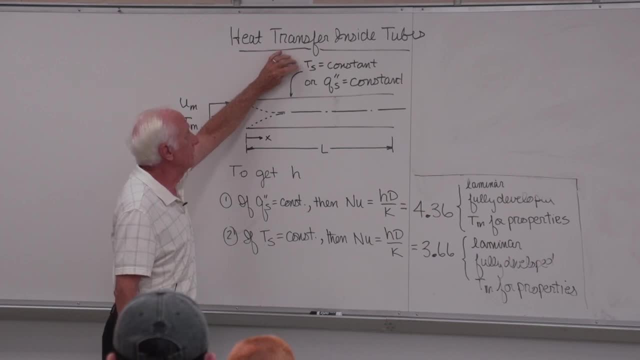 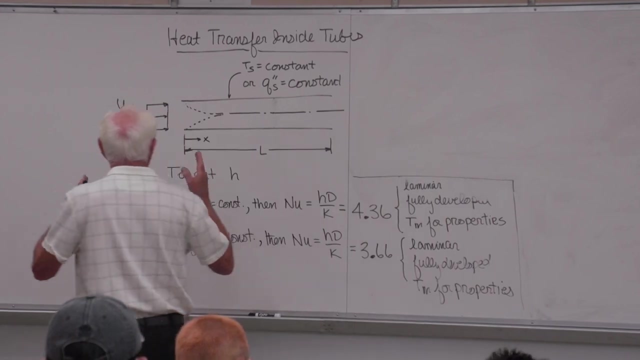 It can either be constant surface heat, constant surface temperature or constant surface heat flux- One of these two guys. Now, so far we've found the X fully developed. It takes a while for the fluid to become fully developed in the tube from a uniform profile. 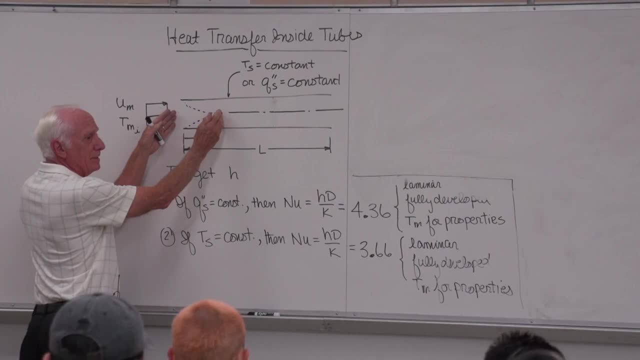 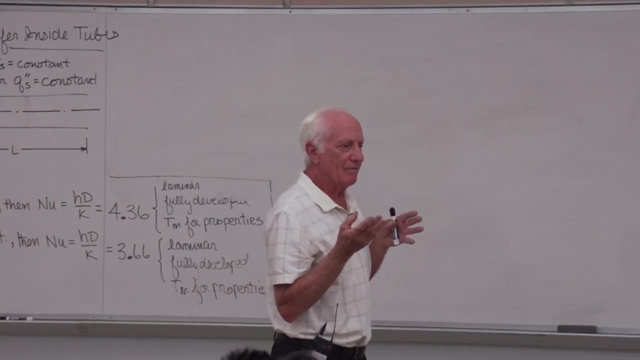 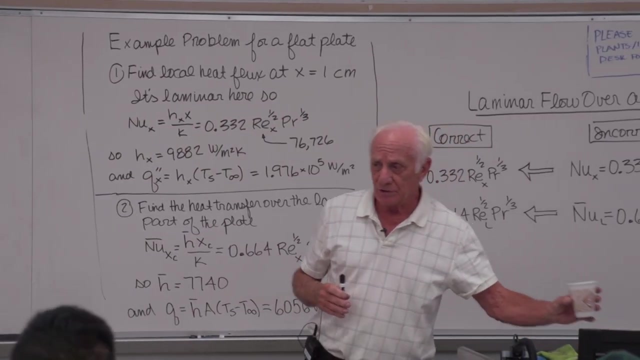 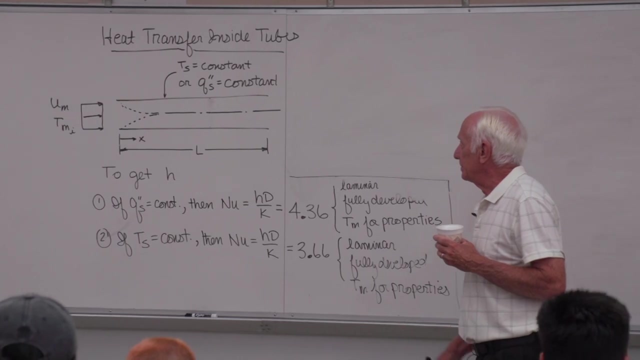 That distance is called X fully developed for velocity or X fully developed for temperature. So last time we put down equations of how you calculate X fully developed velocity and X fully developed turbulent. We also had equations for how the temperature varied with X for those two conditions. 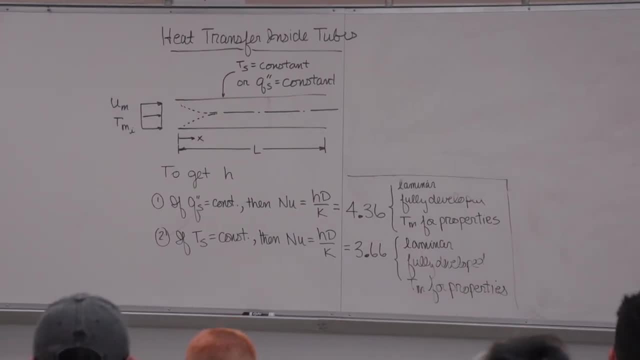 constant tube surface temperature or constant tube heat flux. We had temperature as a function of X, So that's where we left off last time. So now today we get to one of the big things in Chapter 6,, 7, and 8.. How do I find? 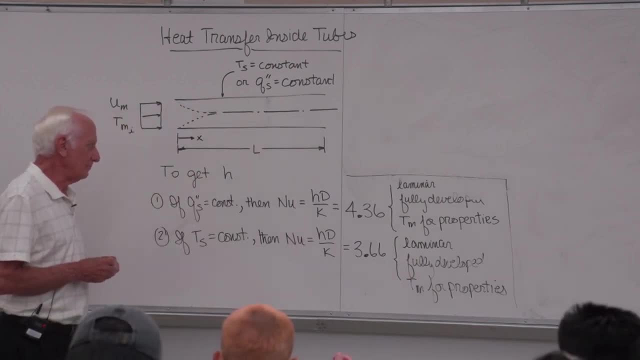 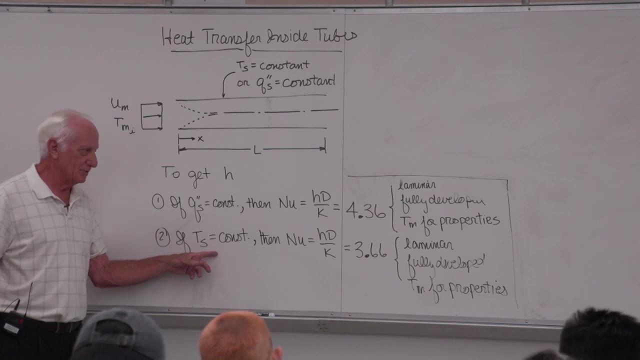 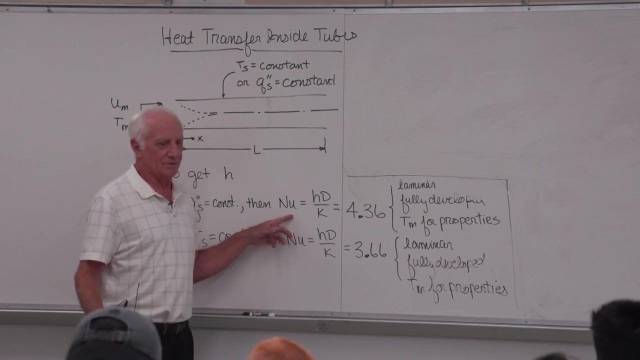 the convection coefficient H. Okay, Two cases, one and two. First one constant wall heat flux, Second one constant tube surface temperature. If it's constant wall heat flux, oh, it becomes ridiculously easy. This it's walked through in. 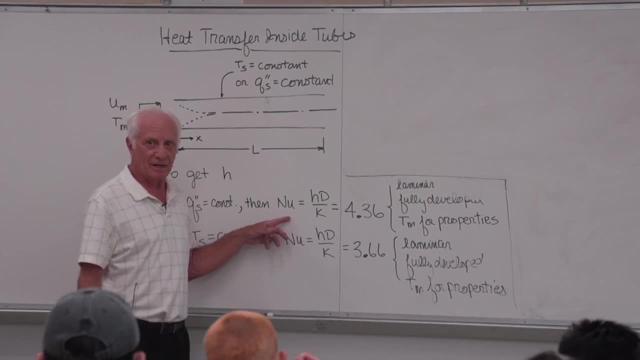 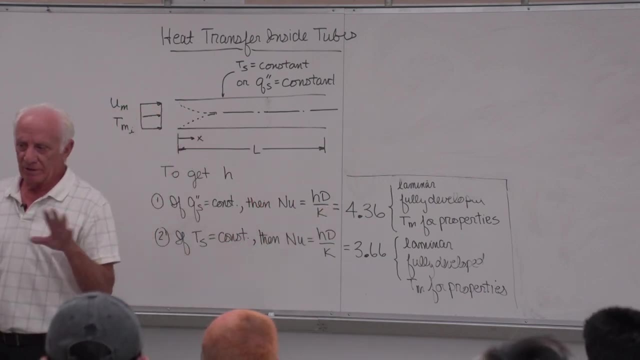 the textbook in a page and a half. We're going to use the result and not go through all the gory details. Nusselt is constant: 4.36.. Just a number. No. Reynolds number no. Prandtl number no. 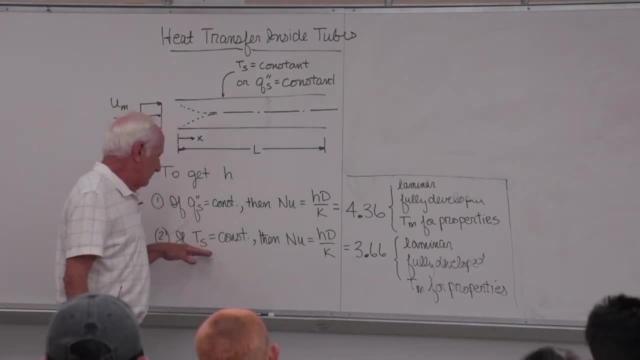 Just a constant 4.36.. If the tube surface temperature is 4.36,, then it's constant. If the tube surface temperature is constant, then the Nusselt number is just a number: 3.66.. No Reynolds number, no Prandtl number, just 3.66.. 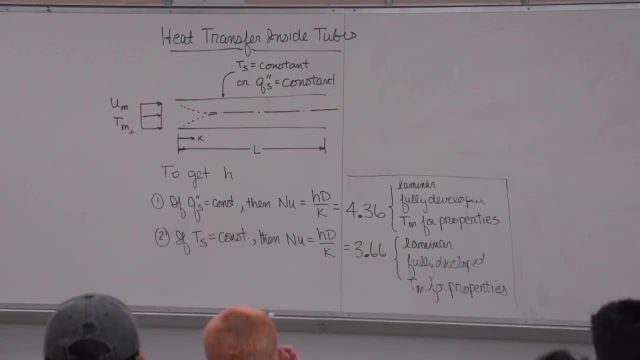 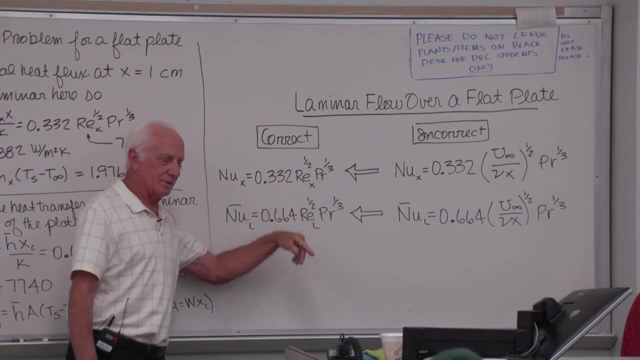 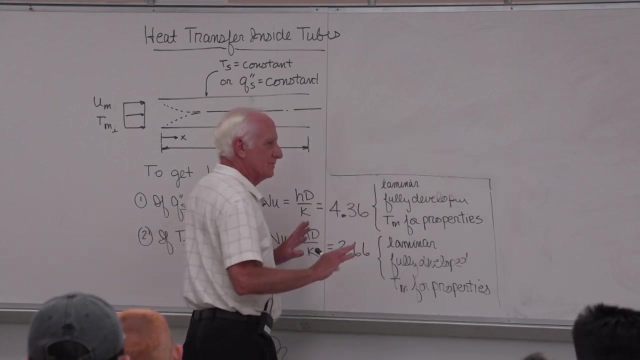 You go back to flow over a flat plate. Nusselt number: it's not a constant, It depends on X right there. Reynolds number In this case for these conditions constant. Now, it's only valid for certain conditions. 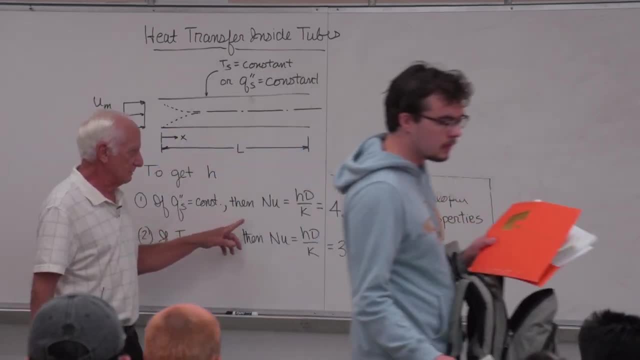 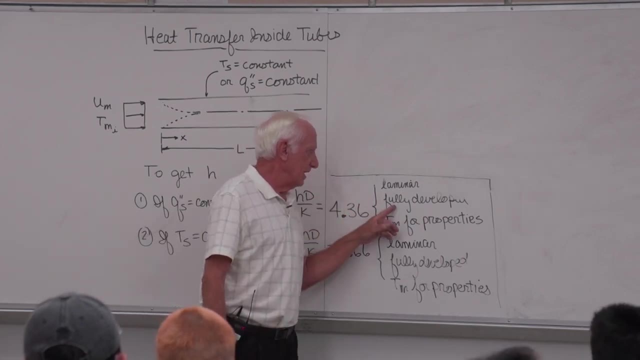 So take the first one. QS double prime is a constant. It's only valid for laminar flow. It's only a constant value if it's fully developed velocity and fully developed temperature and we evaluate the properties at T mean, the mean fluid temperature. 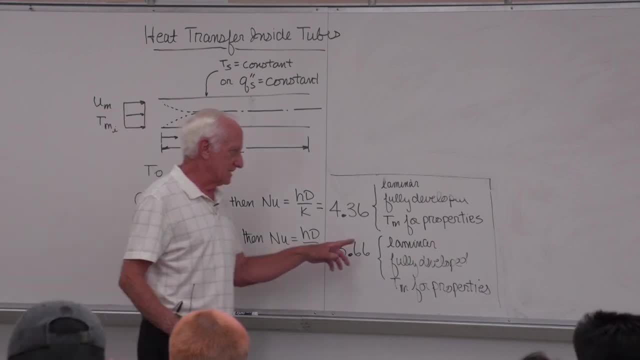 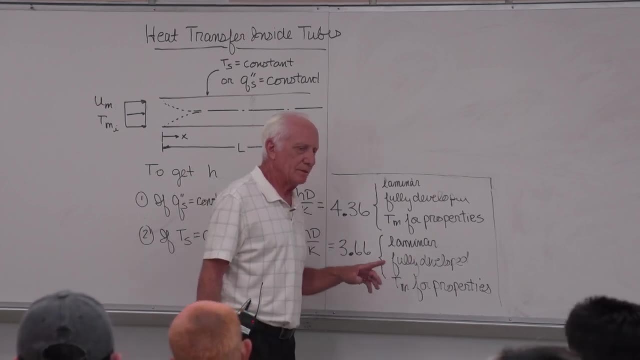 Same thing for a constant tube surface temperature: It has to be laminar flow: It has to be fully developed. velocity, It has to be fully developed. temperature and properties of T mean We'll talk about what fully developed means in just a minute. 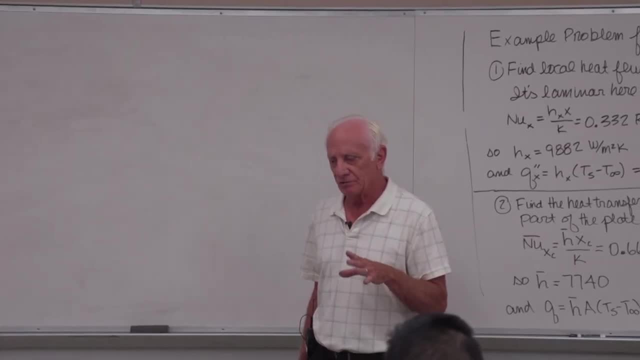 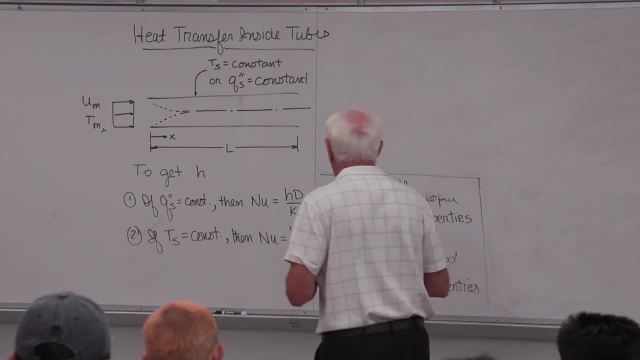 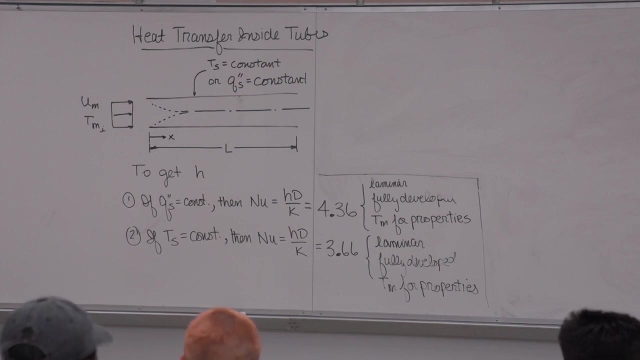 but for right now, those are the conditions that have to be satisfied to use those simple equations. So now we get to what happens if we can't use that particular simple equation. Oh, by the way, before we do that, let's just look at how we find Q. Let's take if Q S double. 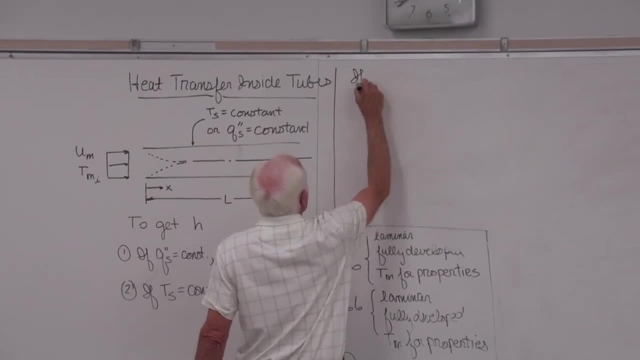 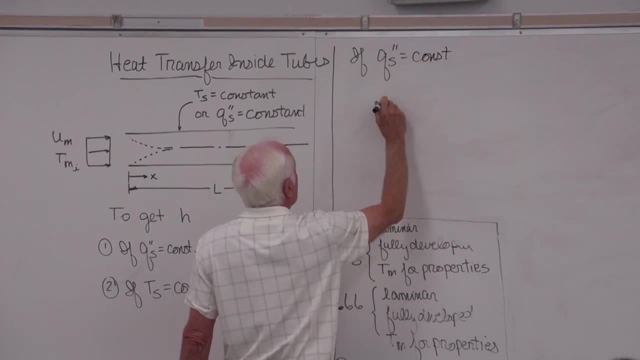 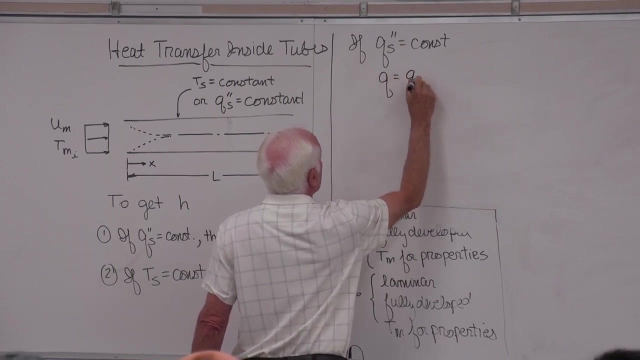 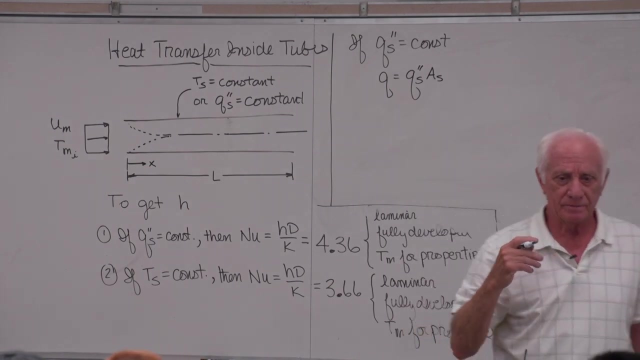 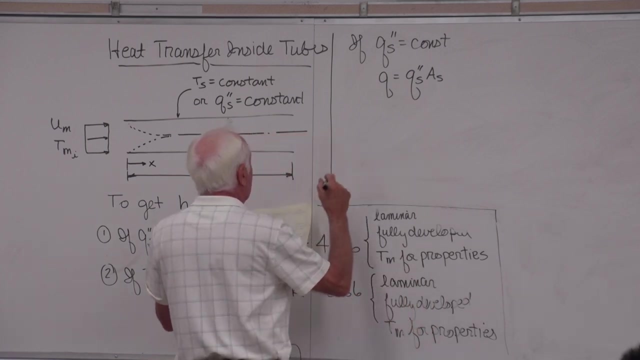 prime's a constant. Okay, then we have Q equal Q S double prime times the area, the surface area of the tube, pi D, L, for instance. Okay, so that one is pretty straightforward. If T S equal a constant, then Q double prime, H delta T L, M. 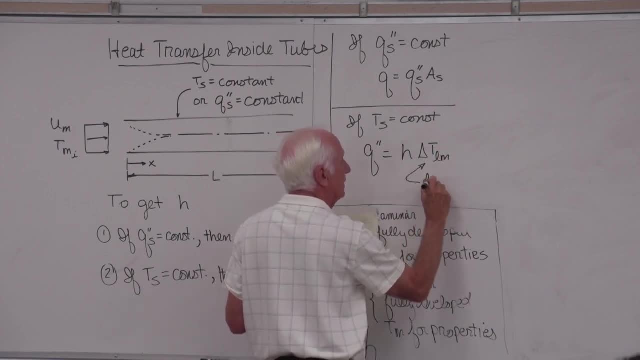 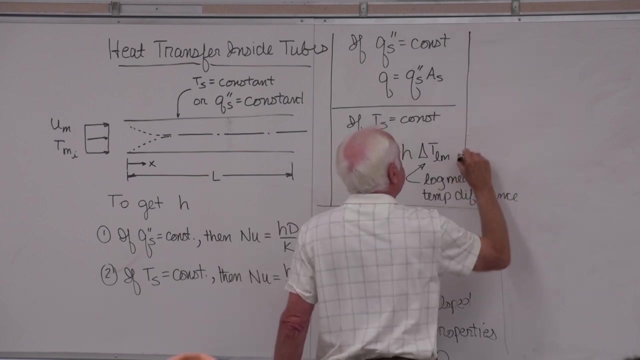 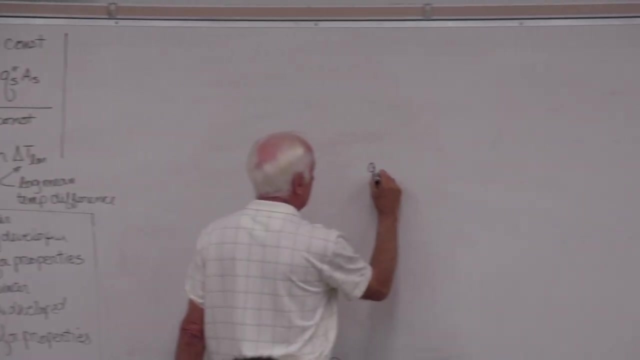 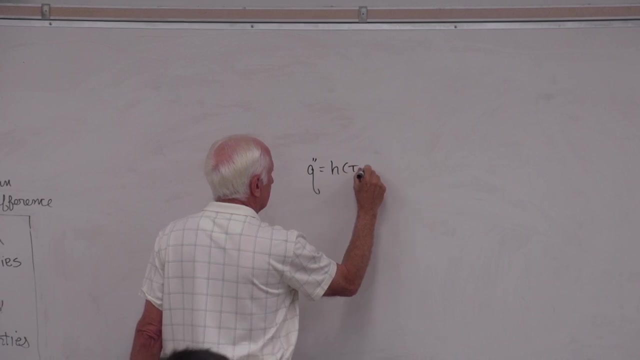 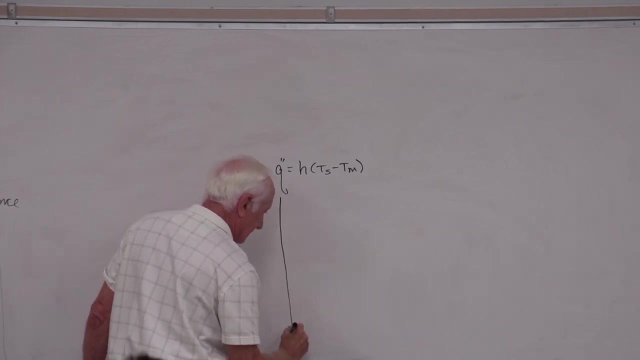 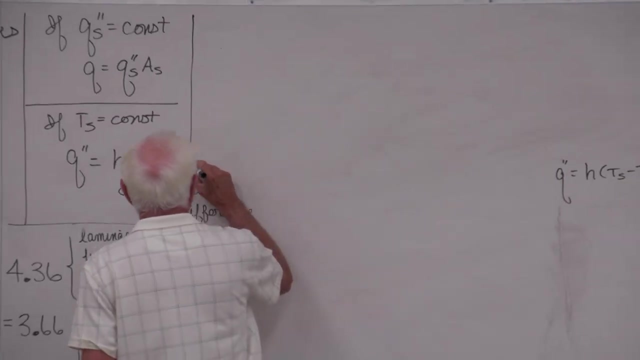 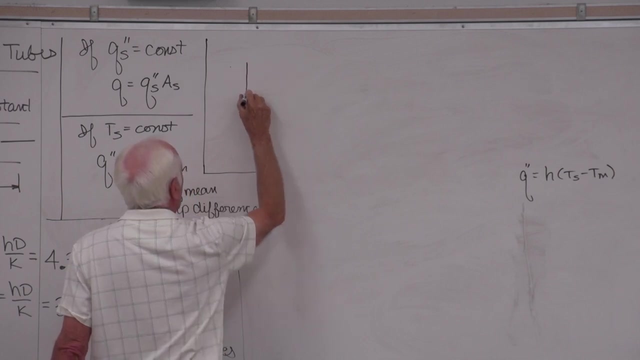 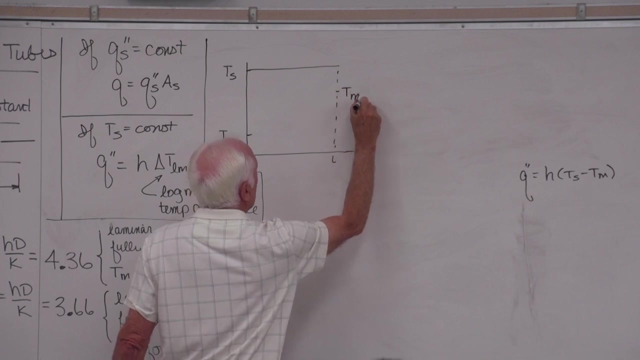 That delta T L M stands for delta T L M, So are the log mean temperature difference. So here's our problem. I'll put it up here, I think, because I want to save it. Okay, So we had that on the board last time. 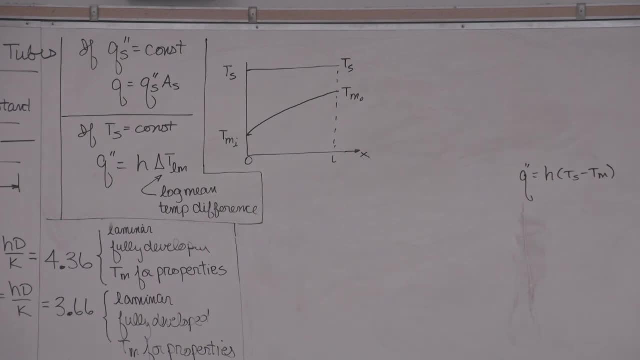 We said. that's how the temperature varies. The fluid temperature varies if the tube surface temperature is held constant. So tube surface temperature is constant with X, But in this case the fluid is being heated. So the question becomes then. here's the equation we've used in the past many times: 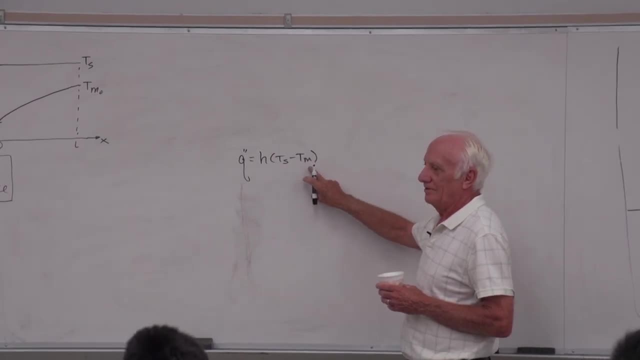 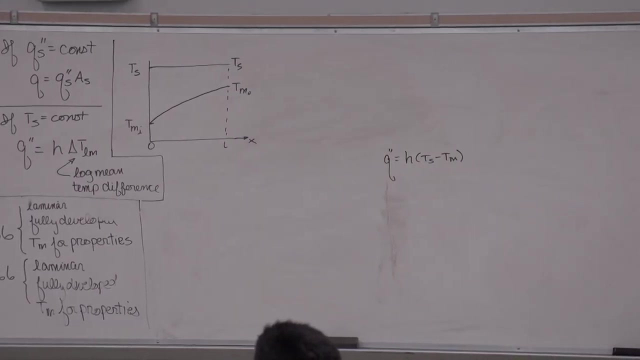 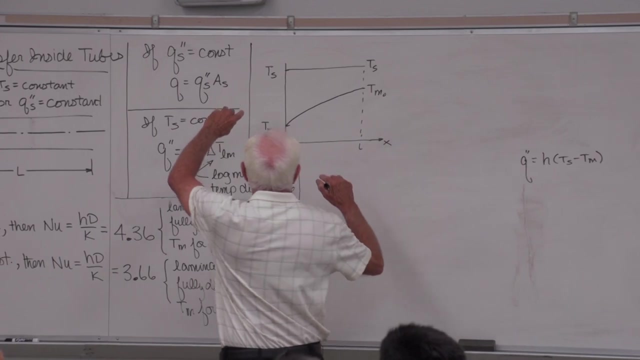 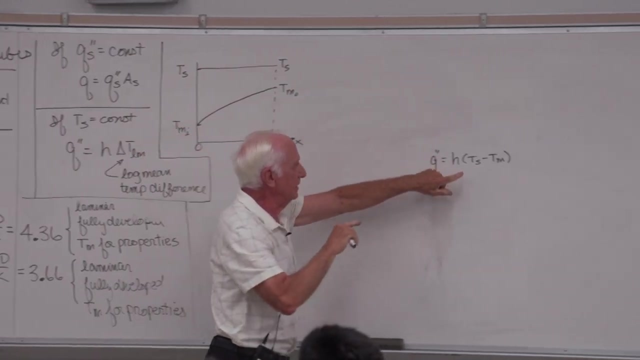 He's a constant. Uh-oh, he's a problem. He's not a constant in that picture. no, So do you put in T S minus T mean in here, Or do you put in T S minus T mean out here? 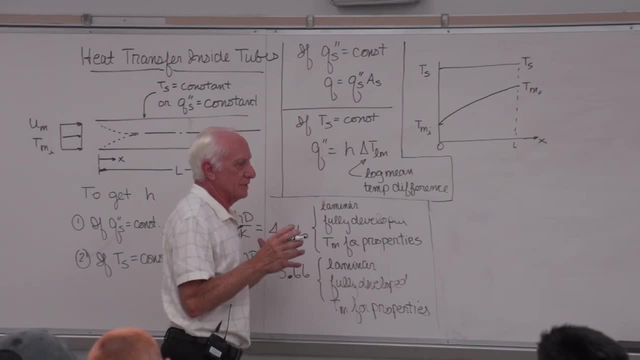 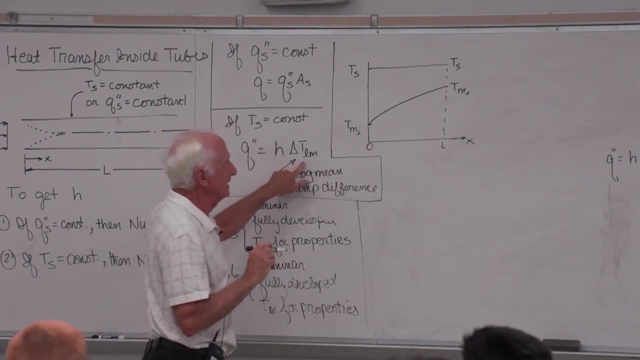 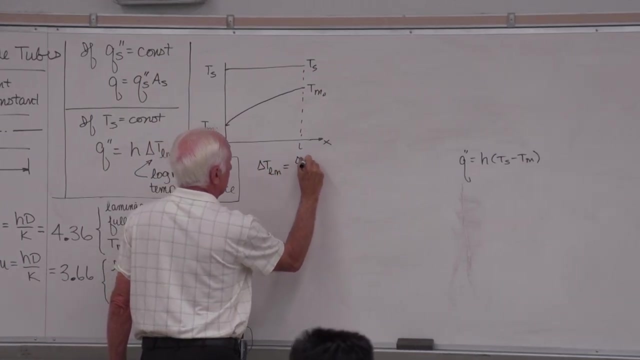 No, neither one. He goes through in the textbook and shows you what you should put in for that. Okay, And what it is is something called delta T log mean Delta T log mean equal delta T out minus delta T in divided by natural log, delta T out over delta T in. 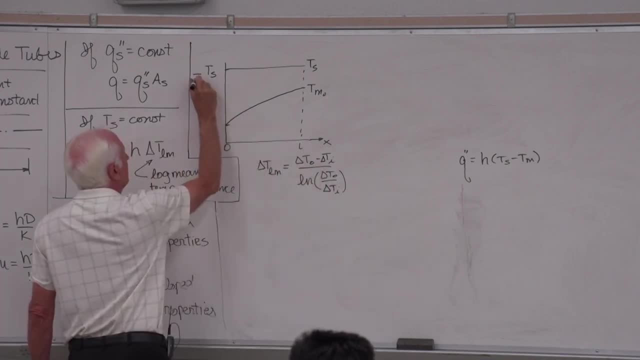 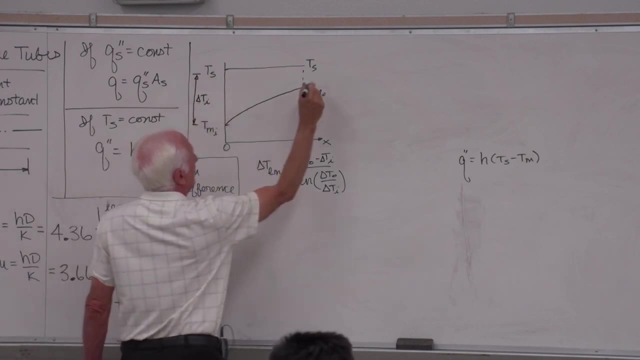 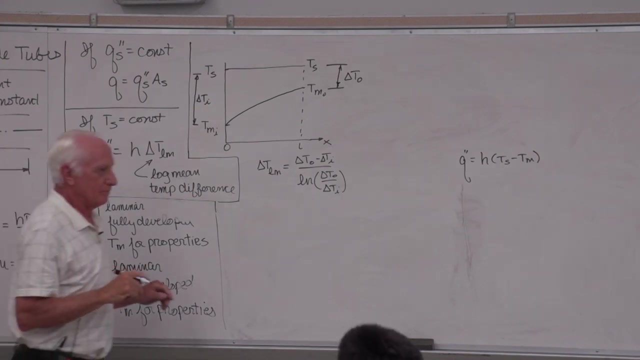 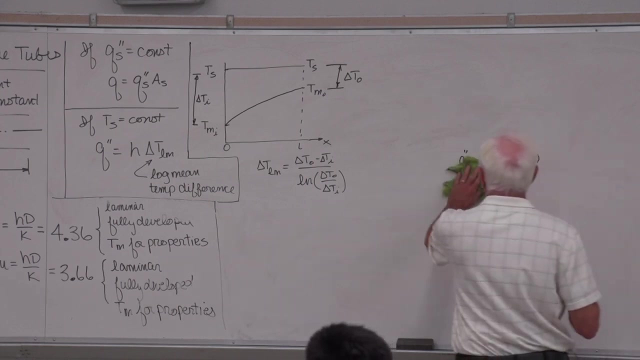 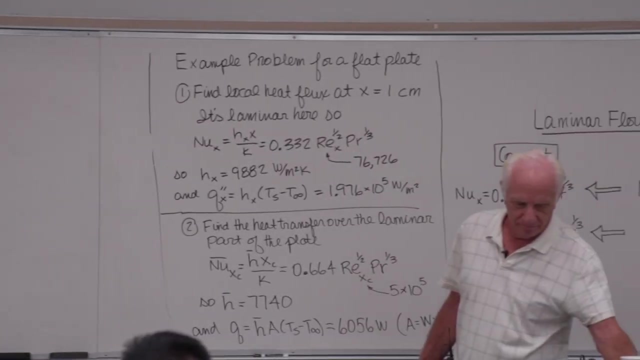 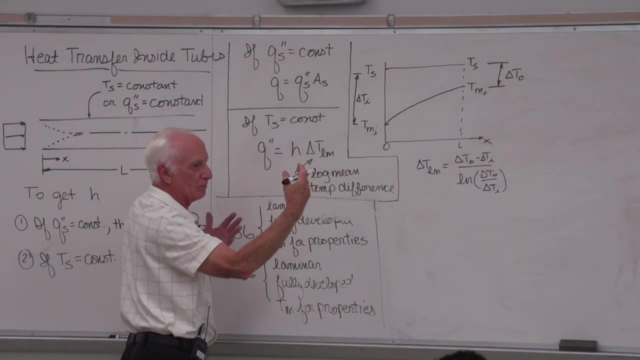 So this is delta T in And this is delta T out. Okay, So now you have that guy, You could find that guy. Okay, All right. So constant mole heat flux if you're given QS double prime. 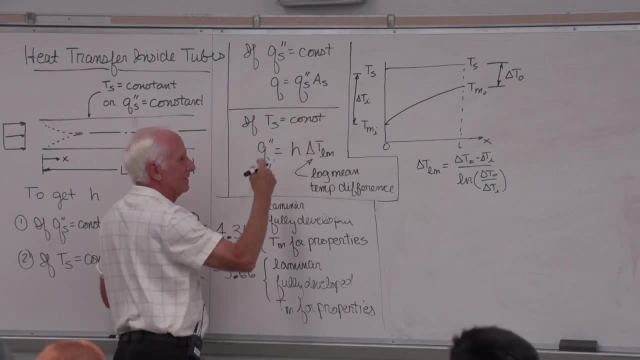 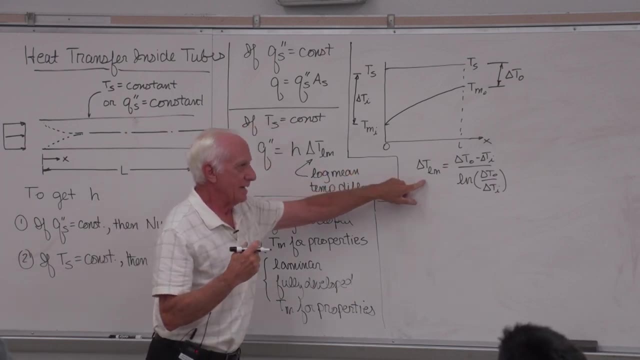 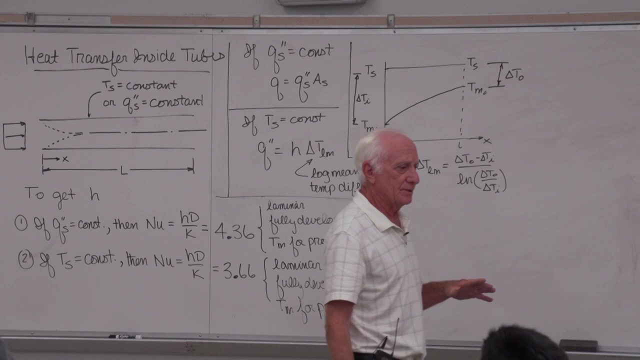 which you normally are. it's pretty easy, of course, That's a given. If the two surface temperature is constant, then you use this guy with that guy. Now you can also use Q equal M, dot, C, sub, P, delta, T, T mean out, minus, T mean in for heating. 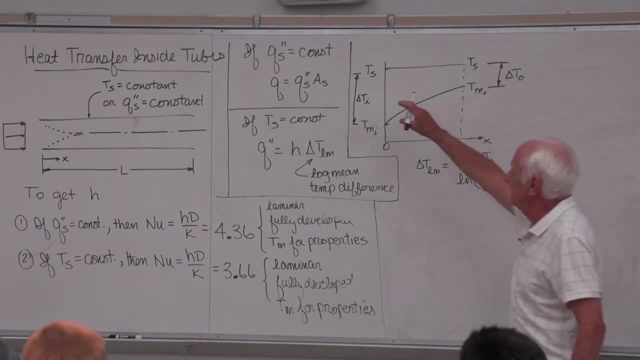 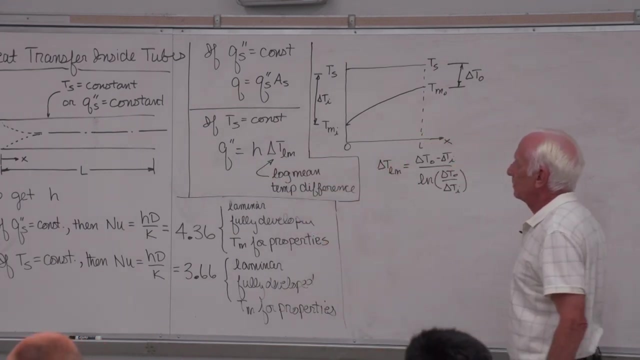 That works for any case. That works for this case and this case. So Q equal M dot C sub P delta T, which is T mean out minus T mean in, works for this case and this case. So really you've got three equations. 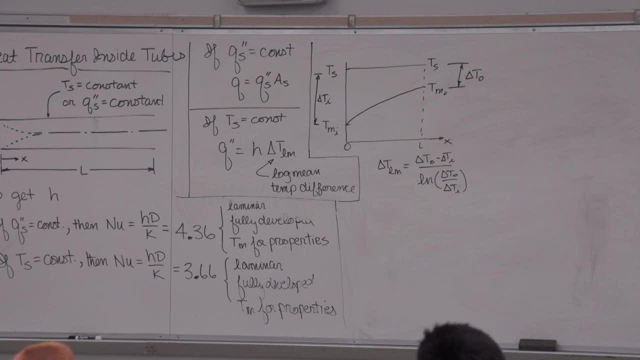 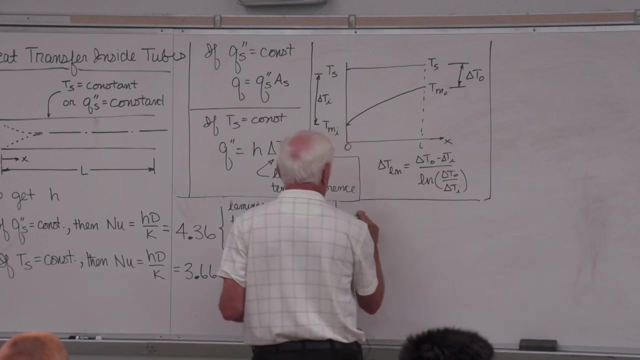 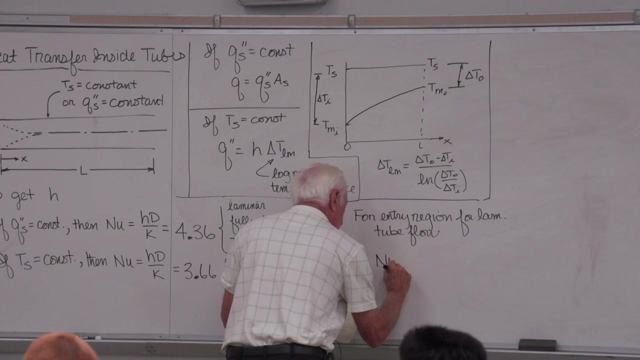 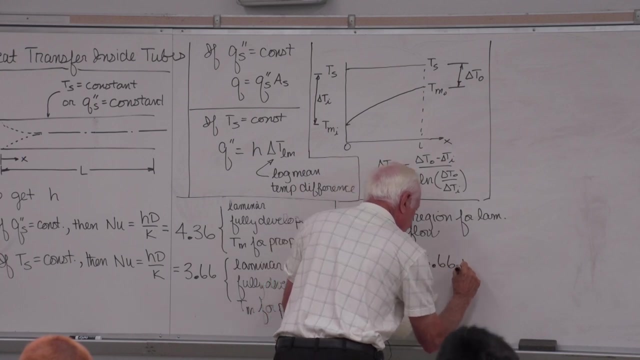 Three equations for Q three. Now, what if it's not fully developed? Okay, Life becomes much more complex. So for the entry region in laminar tube flow, this is the equation we have. 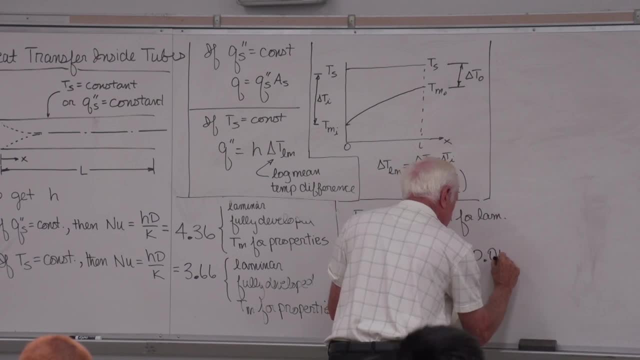 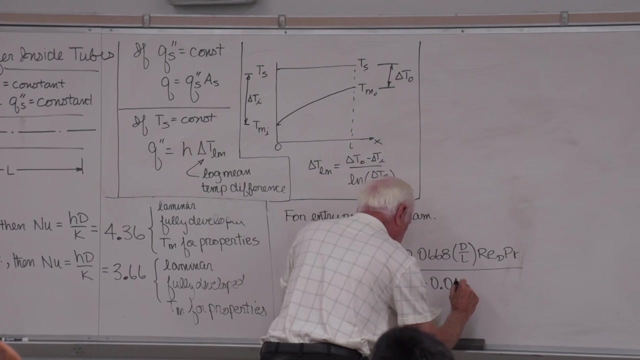 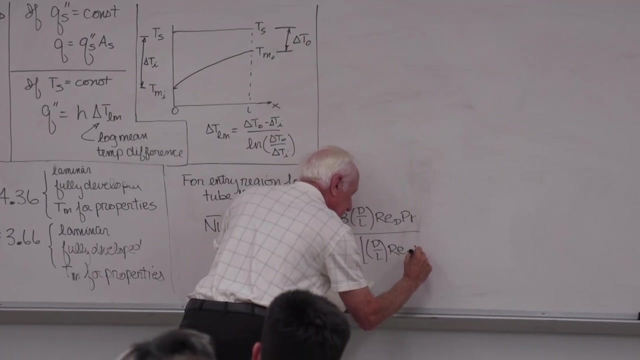 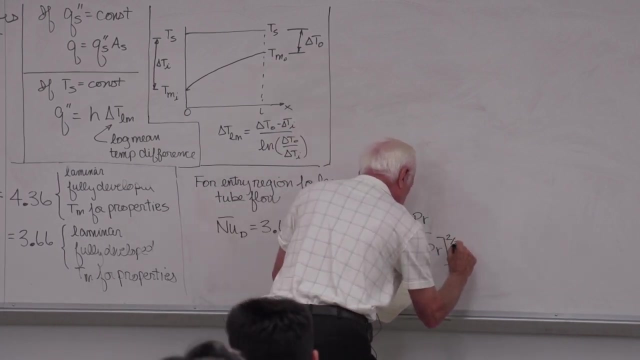 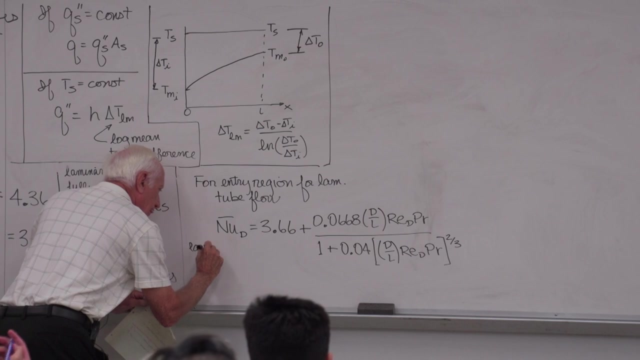 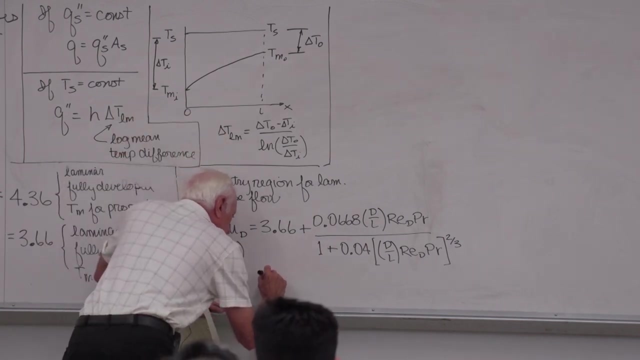 That's the equation in your textbook 857.. So we're going to talk about when do we know if it's fully developed or not? just a minute, But right now. 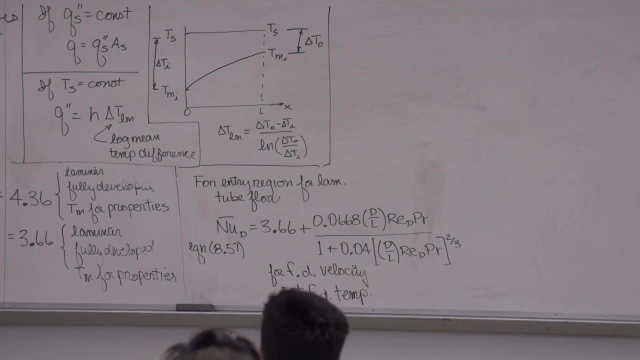 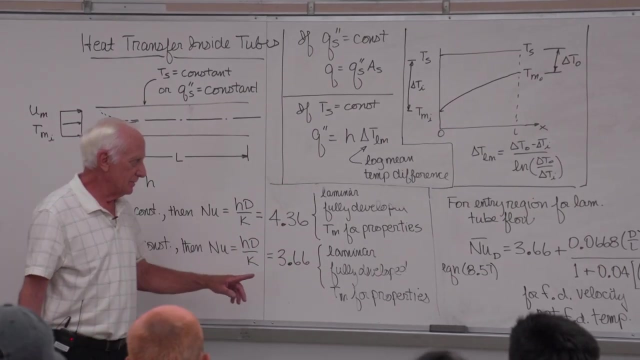 that equation is only good if the velocity profiles can be assumed to be fully developed, but the temperature profiles are not fully developed. Go back over here for these two simple equations. They both are fully developed, both velocity and temperature. You can see the similarity. 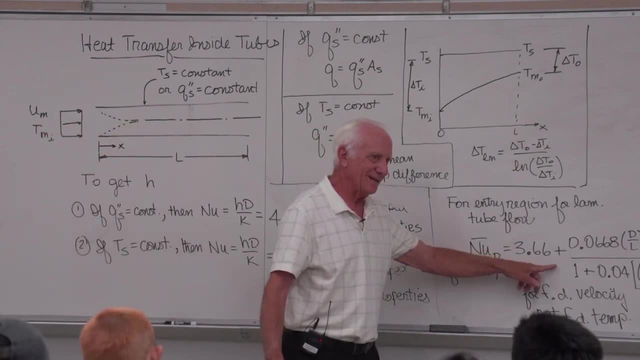 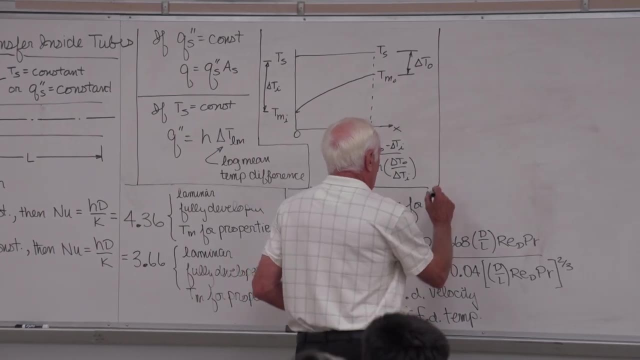 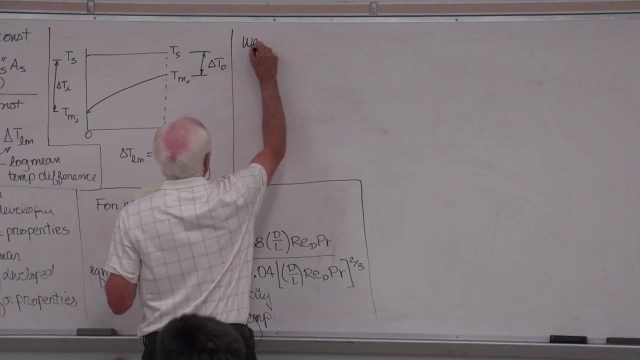 Here's 3.66.. Here's 3.66 plus like a correction factor. So that's what it is: 3.66 plus some kind of correction factor of sorts We also have. oh, by the way, before I forget it, 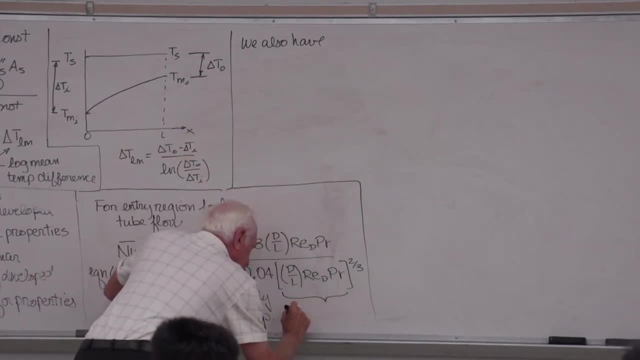 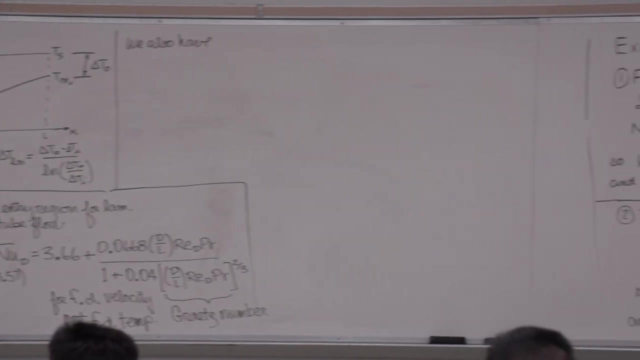 this guy right here in the brackets is called the Grotz number, A dimensionless parameter. again, we engineers love dimensionless parameters, So we just call that guy, rather than D over L Reynolds-Prandtl. let's simplify the world: call it Grotz number. 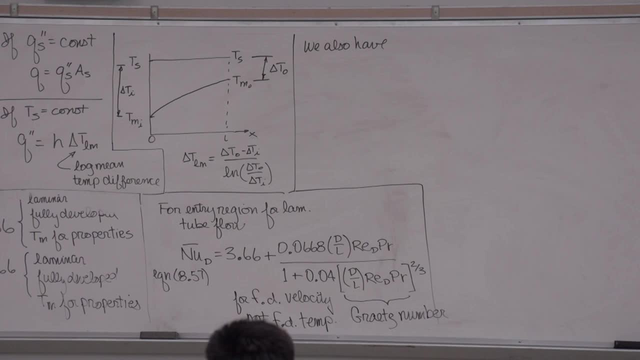 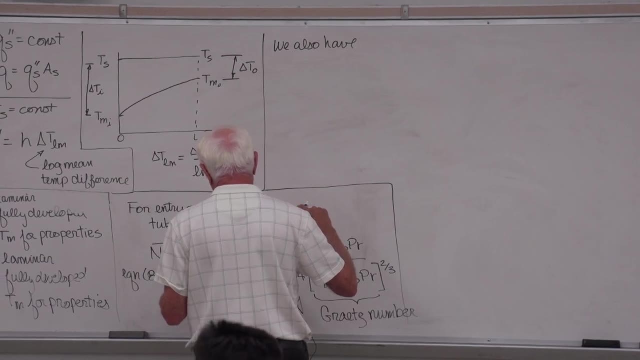 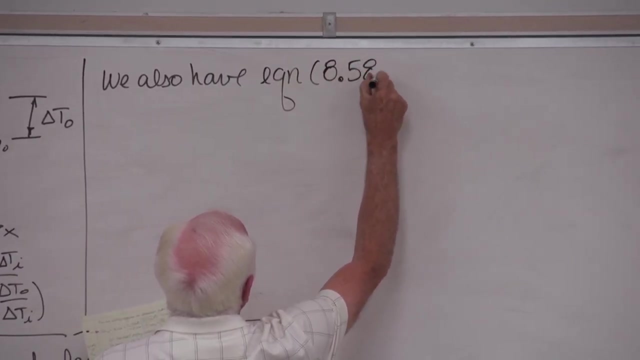 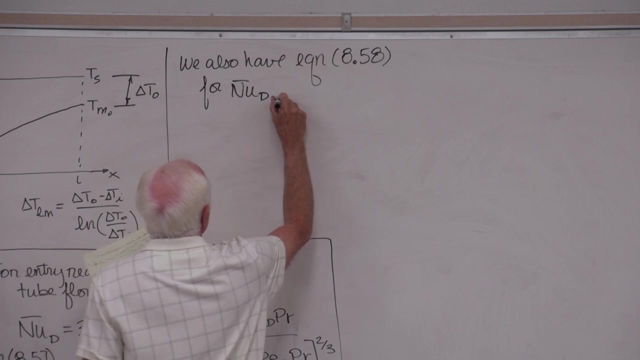 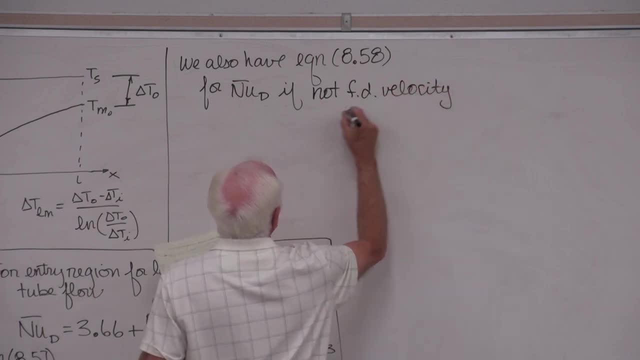 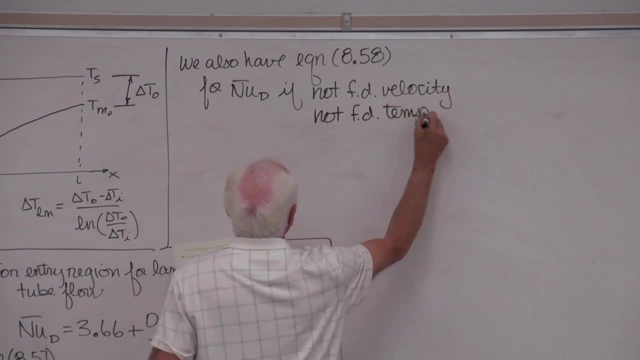 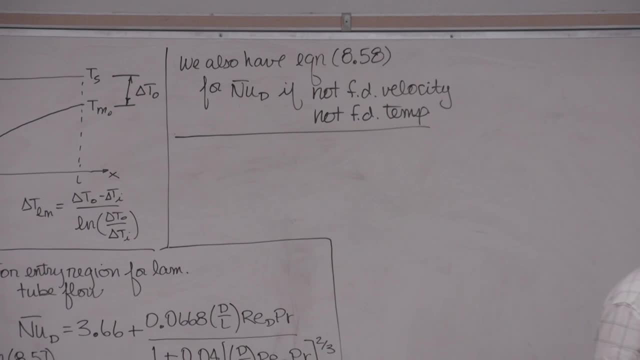 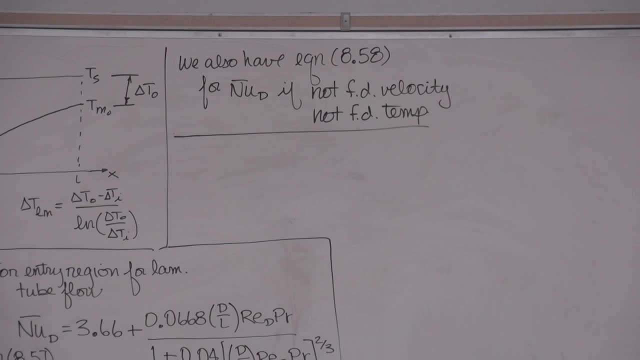 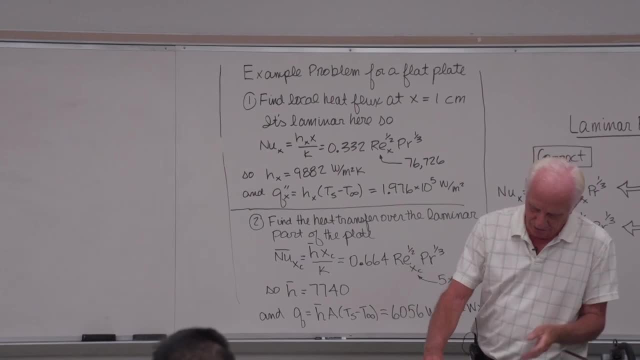 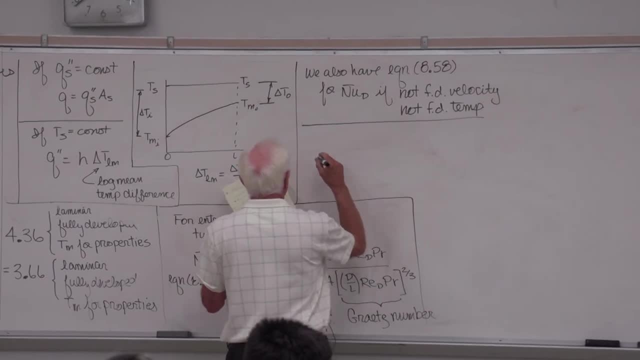 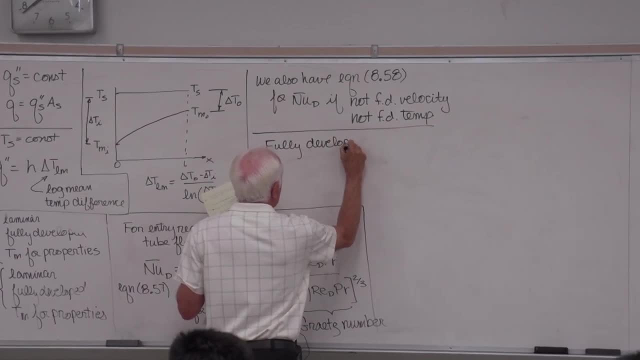 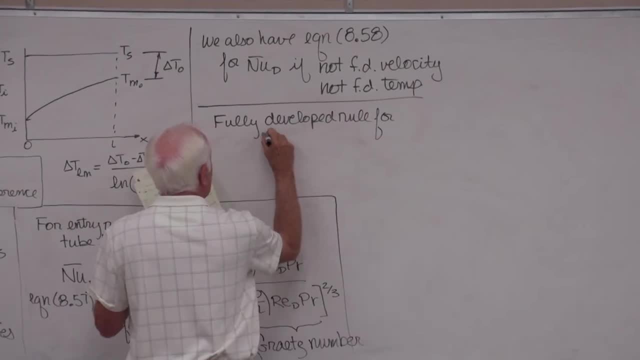 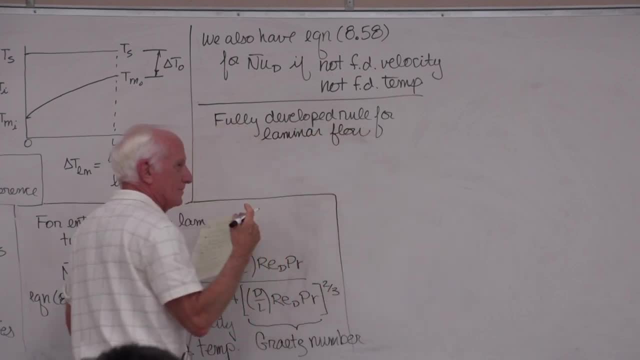 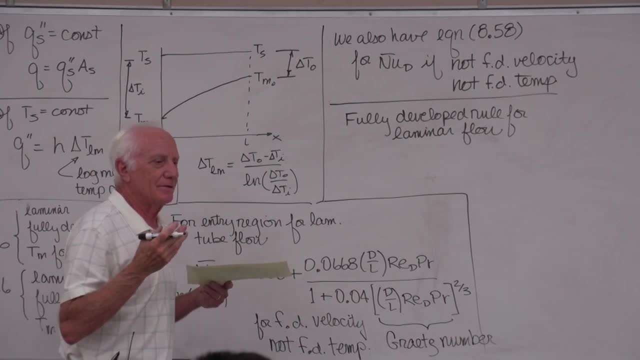 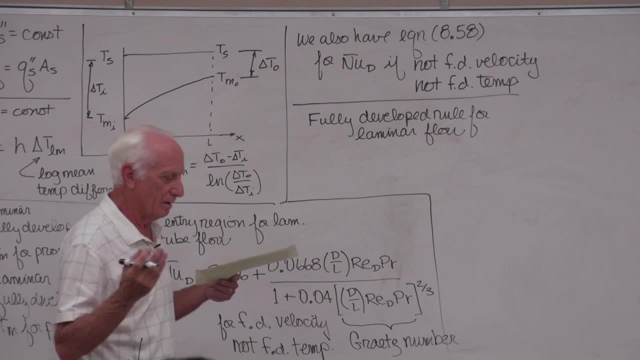 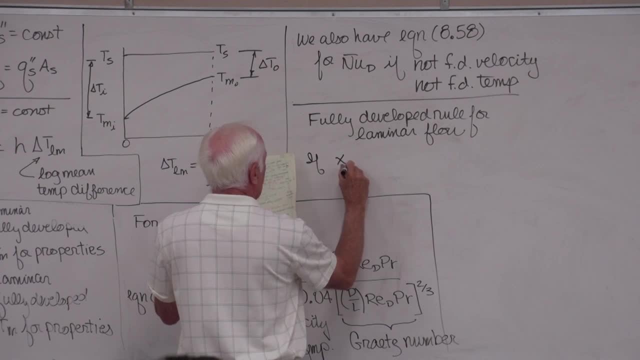 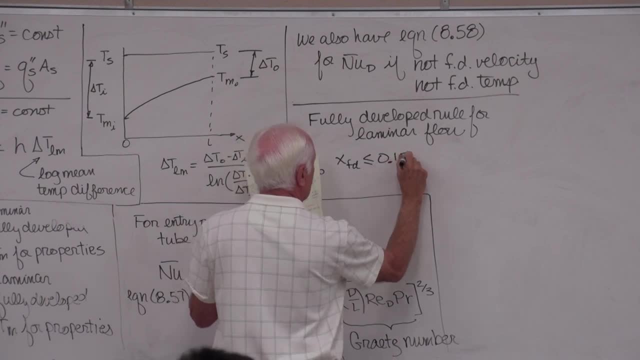 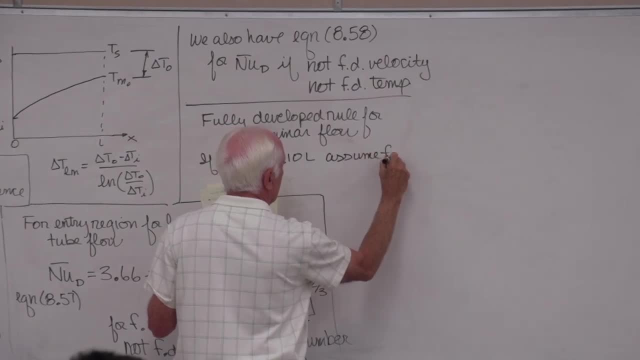 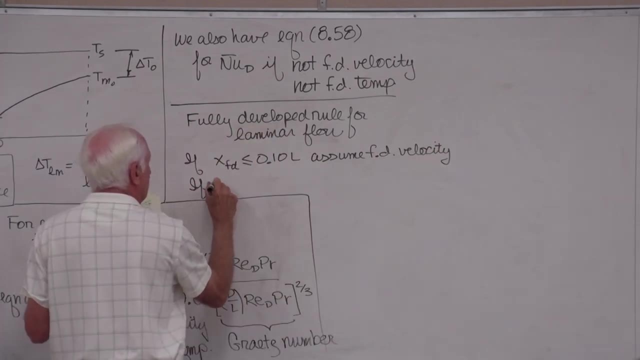 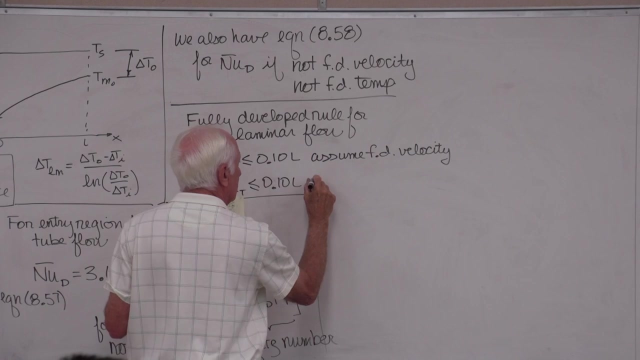 If not fully developed, not fully developed. If not fully developed, not fully developed. If not fully developed, not fully developed. Atint of velocity: If X fully developed temperature profiles less than or equal to 10% of L- Assume fully developed temperature. 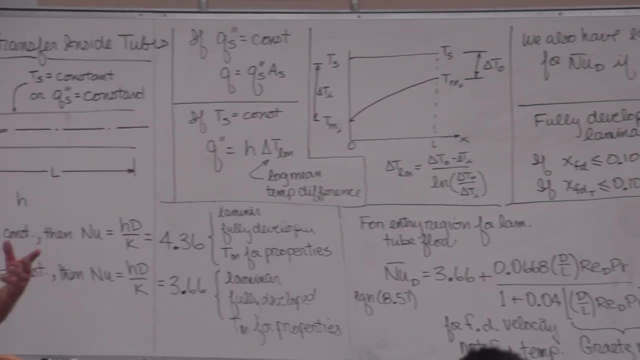 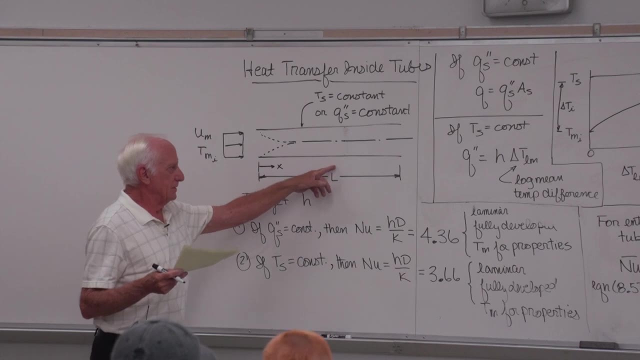 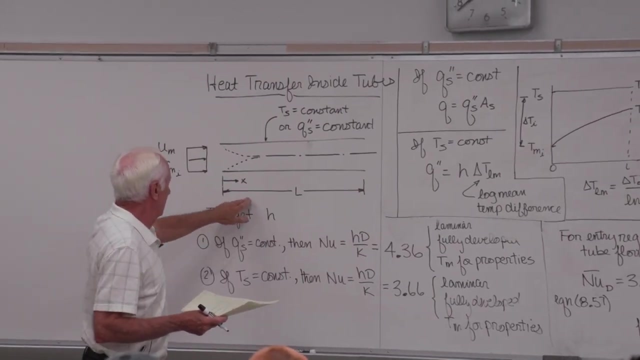 So in a problem like that, you calculate x fully developed. We did that last class meeting. Calculate that. Let's give an example: If L is 10 meters and you get x fully developed, velocity of 0.5 meters, what's the magic number? 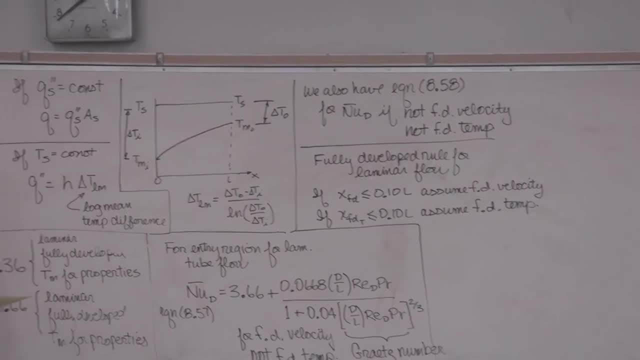 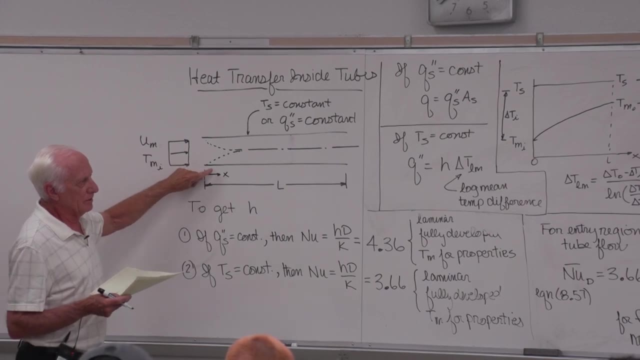 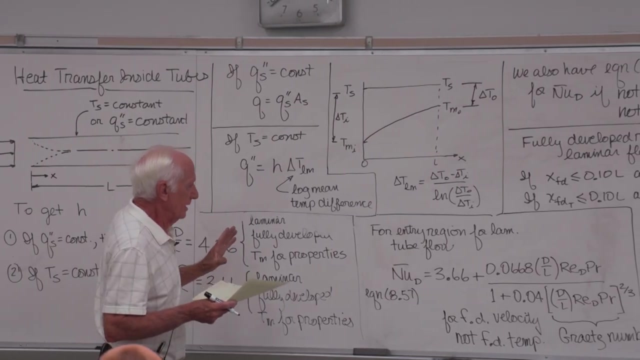 10 percent of L. 10 percent of 10 is one. So if x fully developed velocity is less than one meter, assume it's fully developed. If x fully developed temperature is less than one meter, assume it's fully developed. That's how you answer the question. 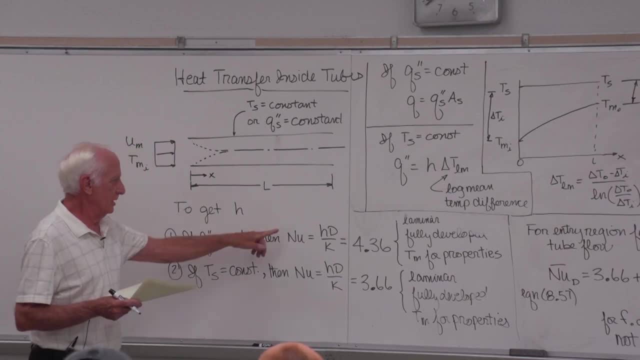 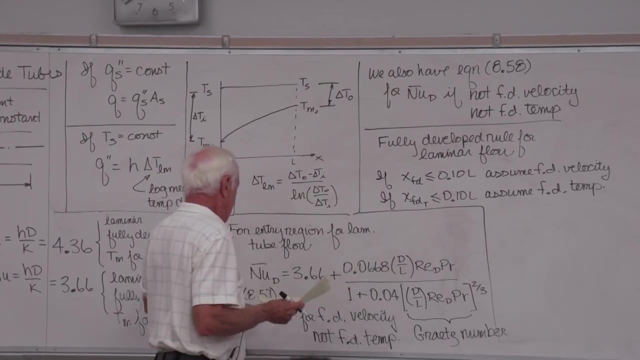 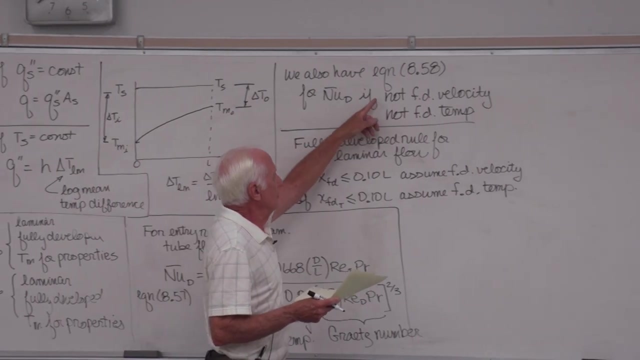 Is the answer yes for velocity, yes for temperature. Here's the two equations. If the answer is here: yes for velocity, no for temperature. here's the equation. If the answer is no for velocity and no for temperature, that's the equation. 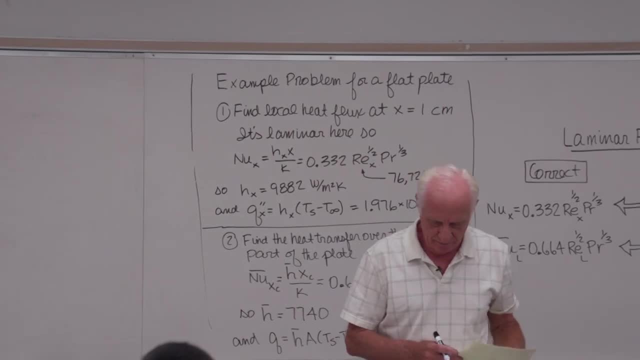 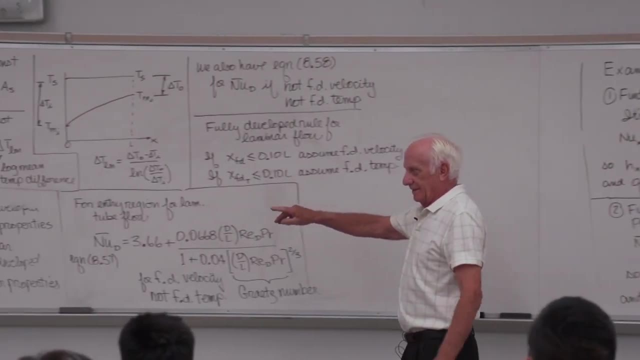 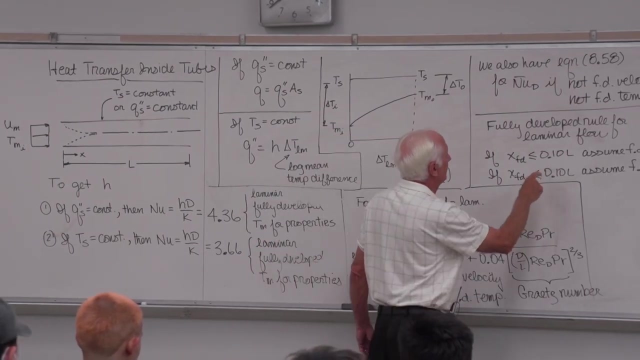 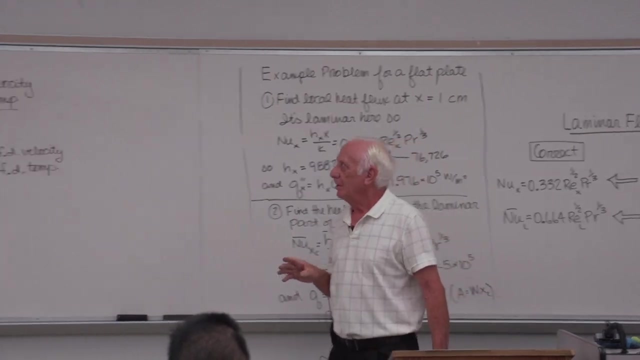 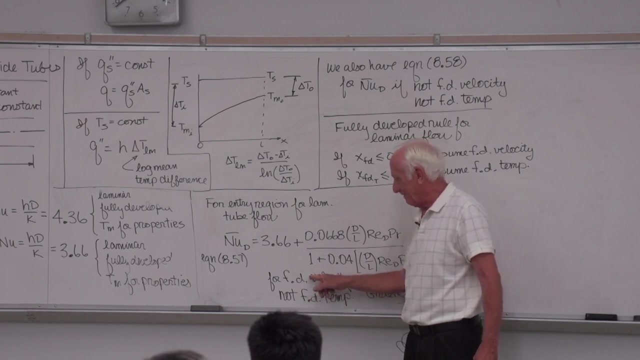 So that's the choices that you have: Yes, yes, yes, no, no, no. So for laminar flow, you've got to answer those questions. You're not going to have no yes. You're not going to have no yes. 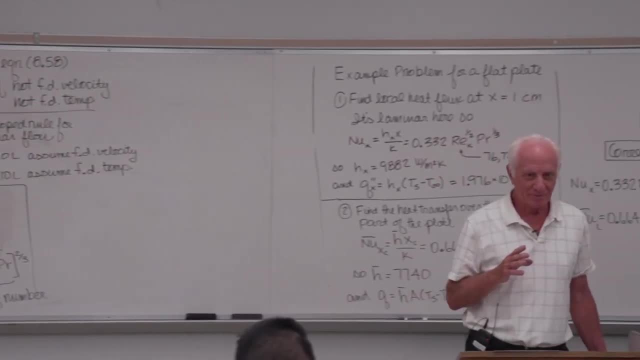 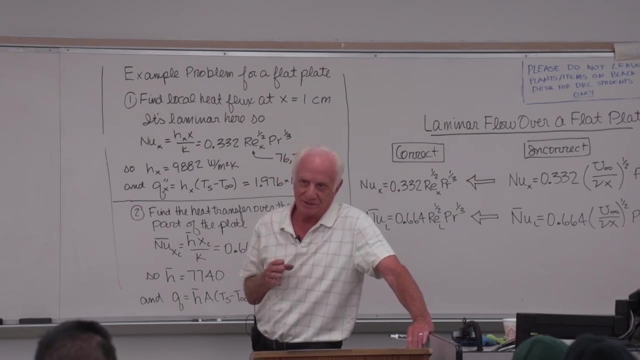 That's for very specific fluids and the textbook mentions, like liquid metals. We don't deal a lot with liquid metals: liquid potassium, liquid sodium. Some nuclear power plants run on liquid metals but they're far and few between, So we don't even consider that option. 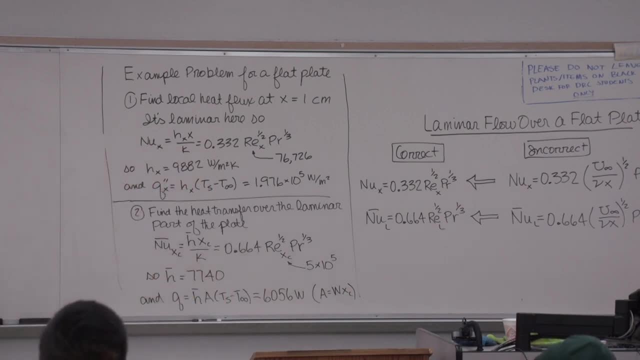 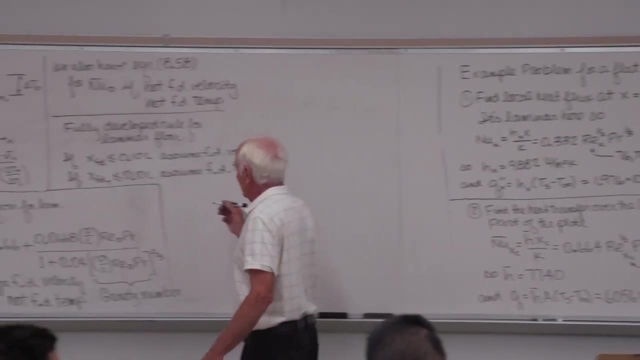 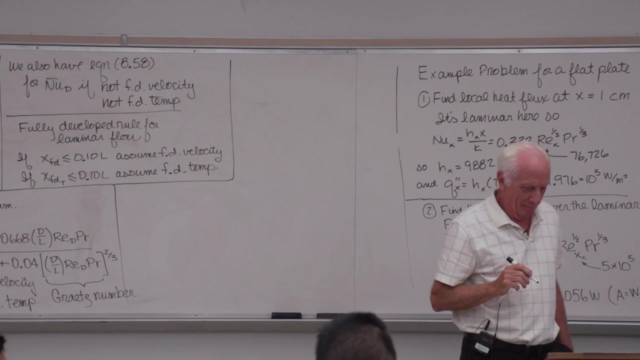 So there's no option over here Of no, yes, forget that one. There's only three options for the fully developed: Okay, So that's all the rules, then, for laminar flow. Now turbulent flow. Okay, I'll put it here. 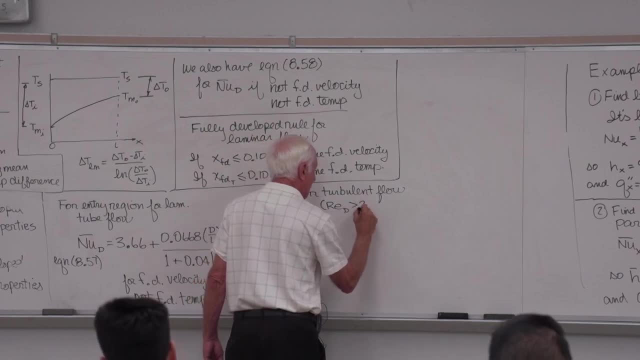 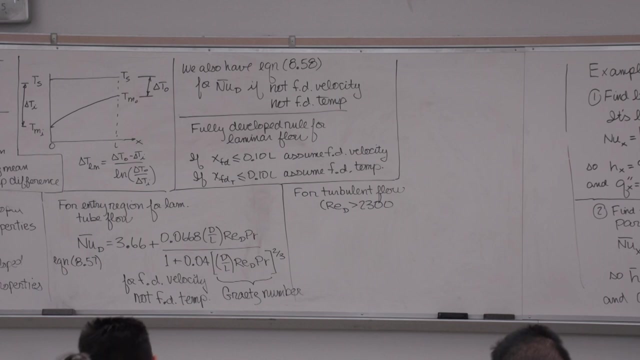 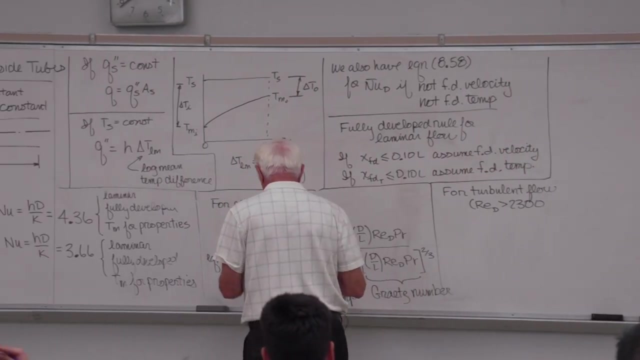 For turbulent flow. we've got a couple of choices. Well, no, I'll just put down the one. I think we'll live with that one. Let's see if I've got my turbulent flow here somewhere- Turbulent flow, just so you know too. 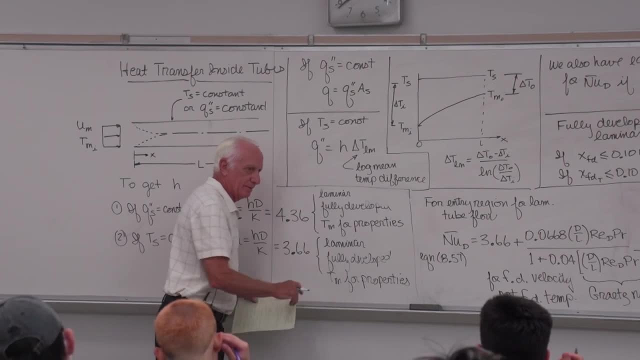 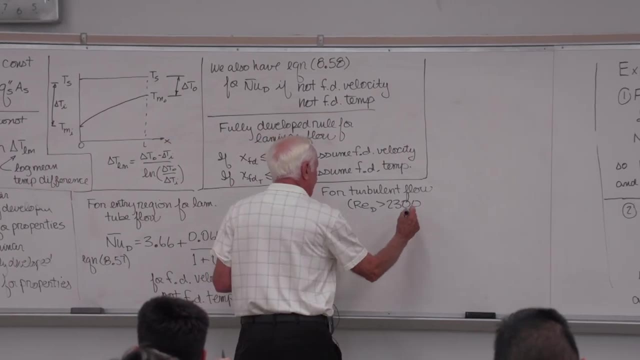 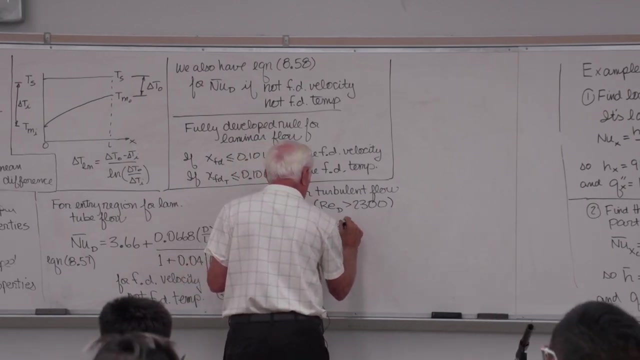 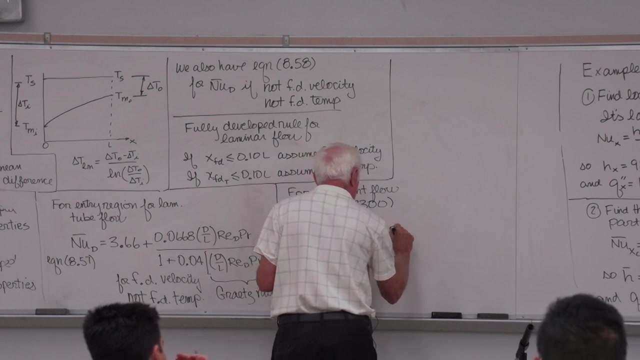 all these guys, every equation so far. properties at T mean the fluid temperature, properties at the fluid temperature: Obviously it's the fluid. Okay, Nusselt d bar, Let's see, Okay, Let's see. So survey that. 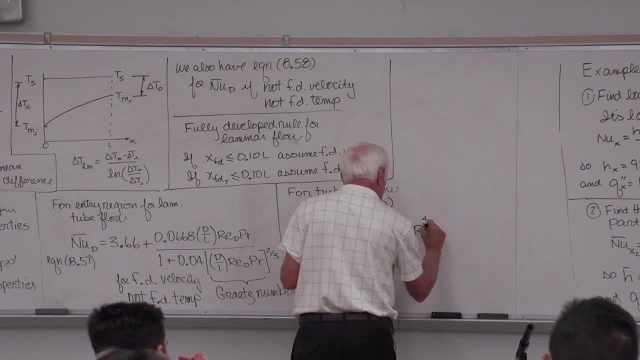 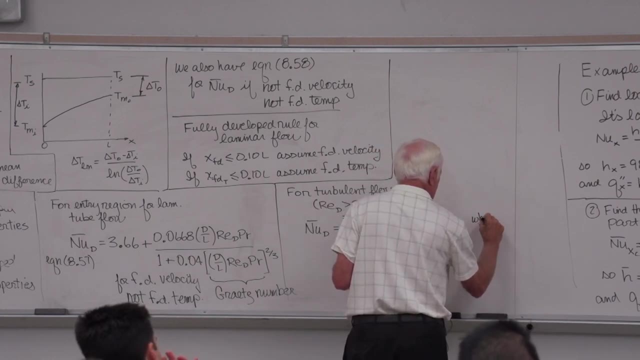 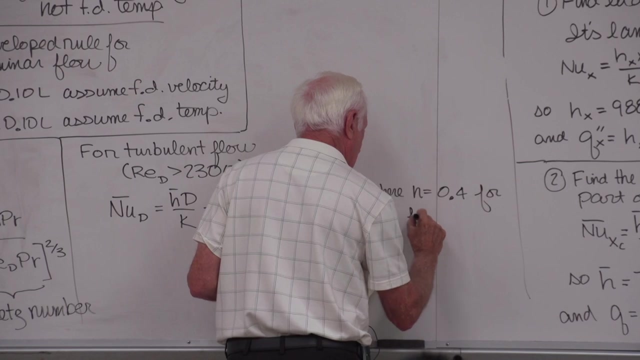 Okay, Let's do that one, Let's do that one. Okay, Okay, Let's take the. let's do that one then, Okay, Let's just go through that. Okay, Okay, Okay, okay, All right, let's do that one. 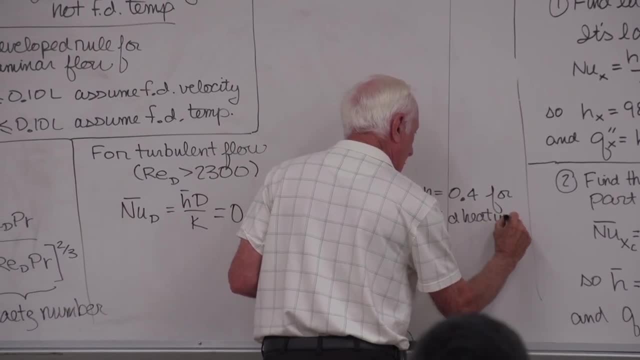 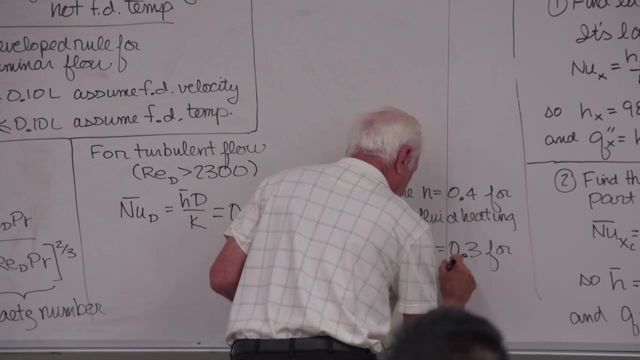 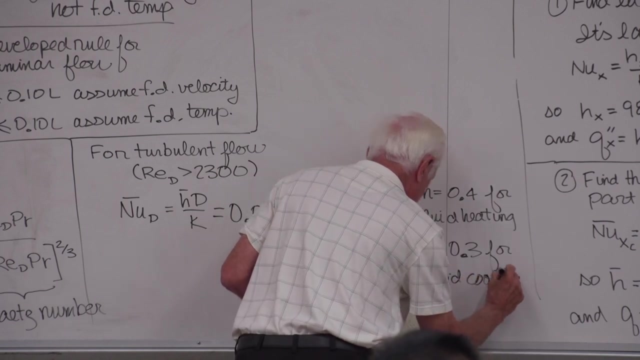 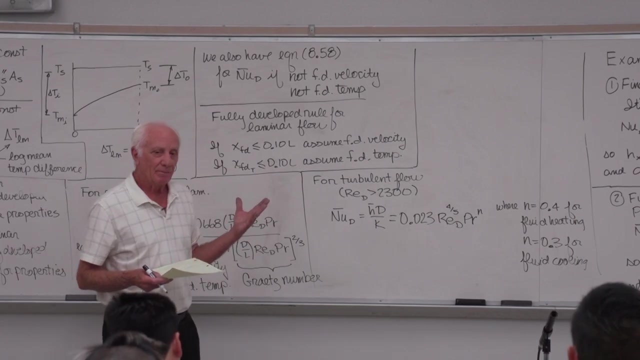 All right, It has the typical form of the Nusselt number and the Reynolds number. Nusselt is a constant times Reynolds number raised to a power times a Prandtl number raised to a power, But in this case the power on. 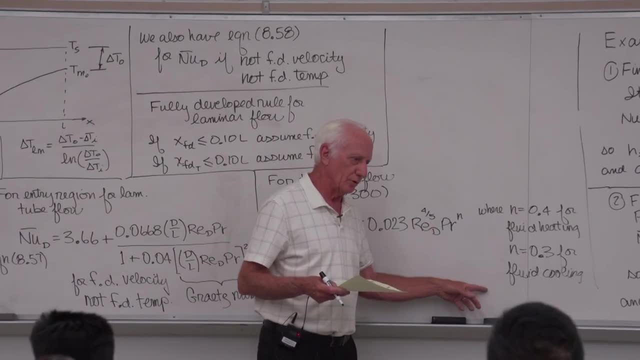 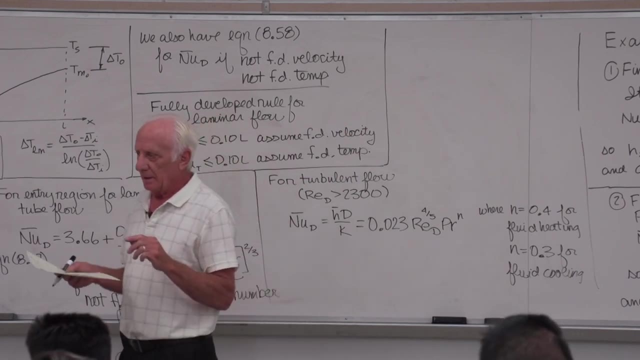 the Prandtl number depends on if the fluid is being heated or cooled. If the fluid is getting hotter as it goes down, the tube N is 0.4.. If the fluid gets colder as it goes down, the tube N is 0.3.. 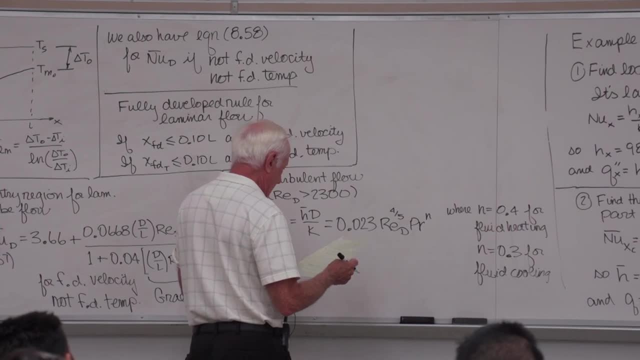 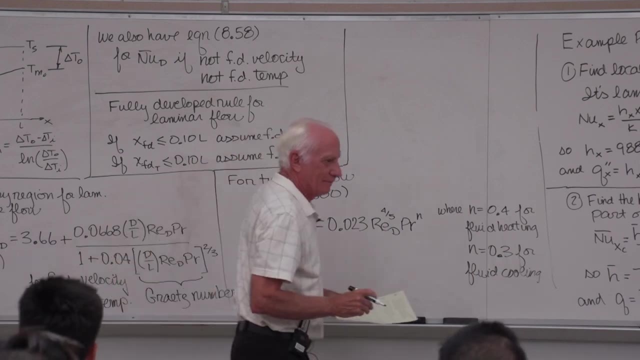 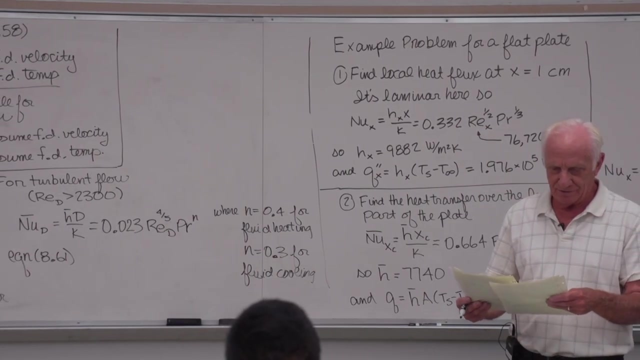 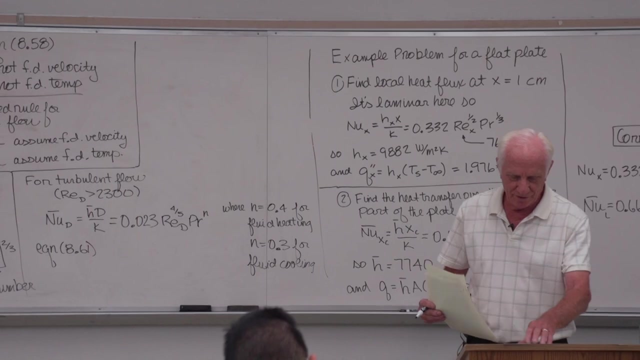 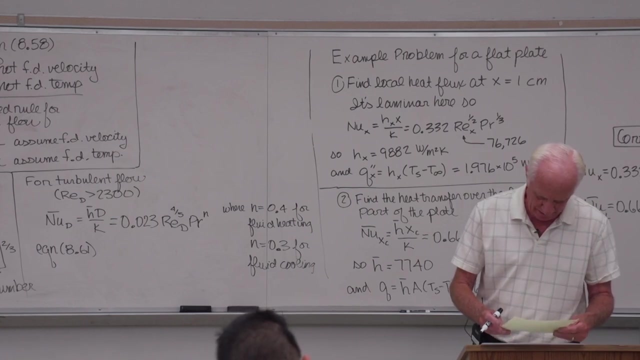 Equation 861.. And of course, the author also puts a qualifier in there. Oh, by the way, all these correlations are within 25 percent, So don't think they're perfectly exact. They're not within 25 percent. Okay, So now there is another equation. 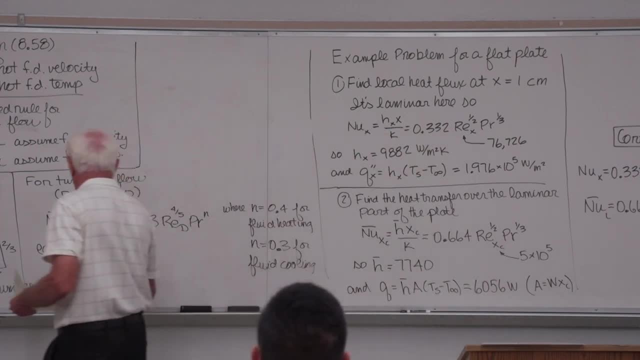 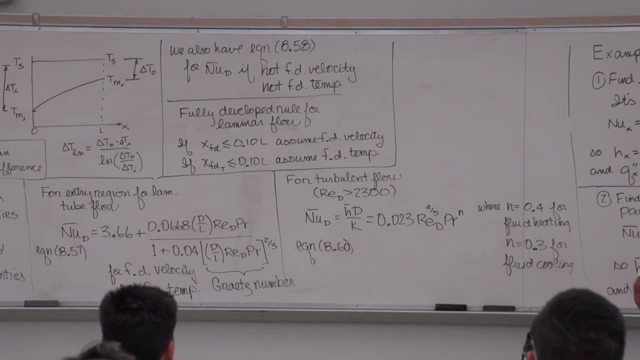 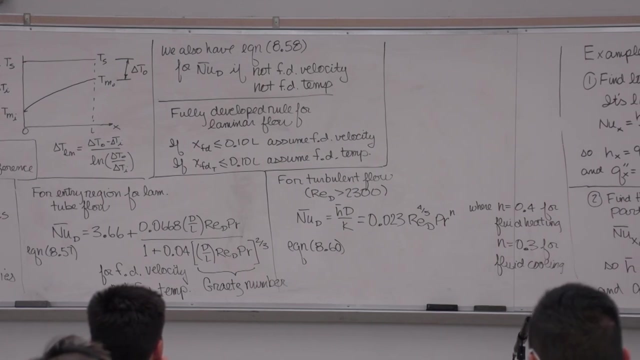 I'm sorry, that's the equation 860, not 861.. There's another equation, 861, which covers a wider range of properties, Prandtl number especially. But we're not going that way, We're going to just use: 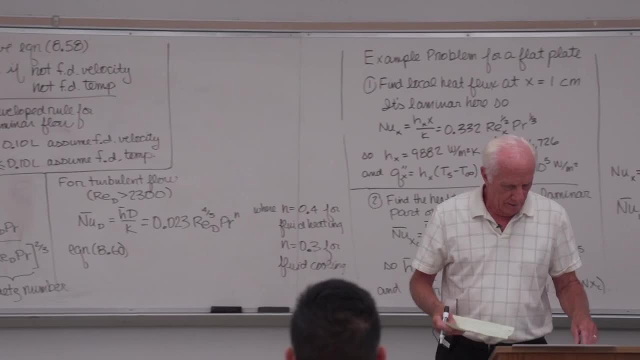 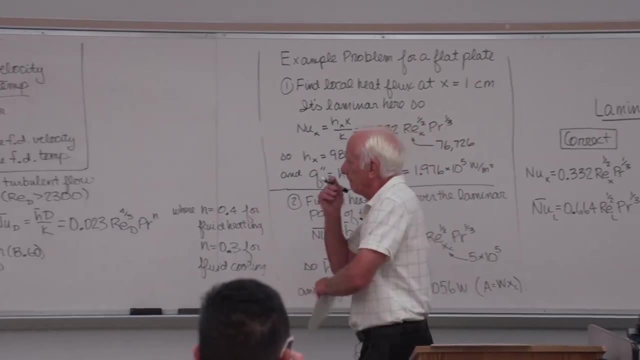 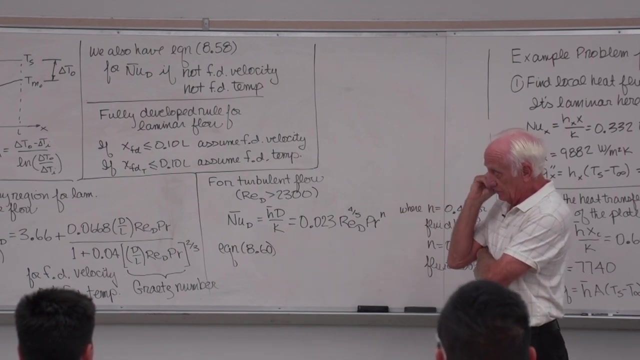 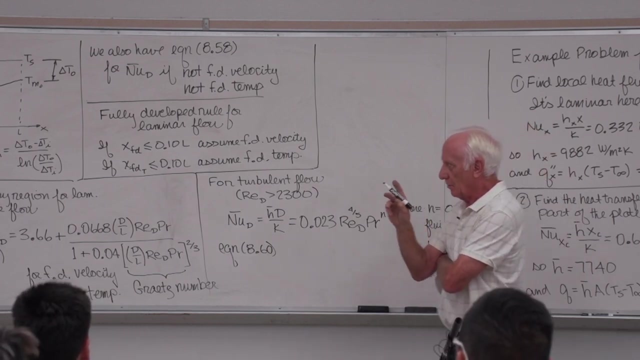 this one equation for turbulent flow. Now, does it, does this equation matter if it's constant tube surface temperature or constant surface heat flux? No, it works for both. One equation works for both. You don't need to ask the question. 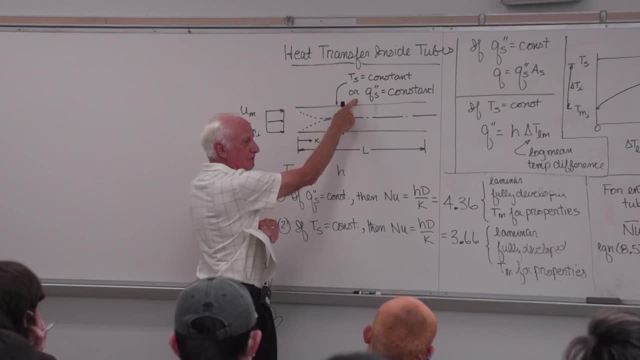 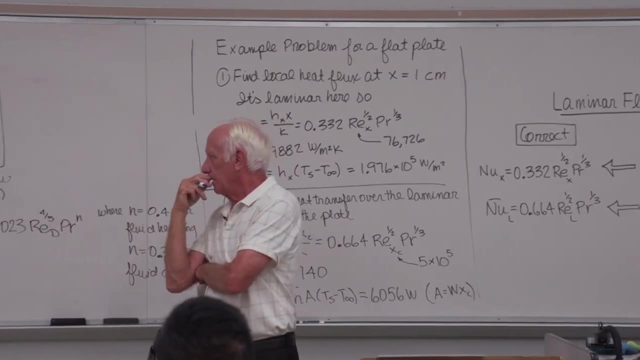 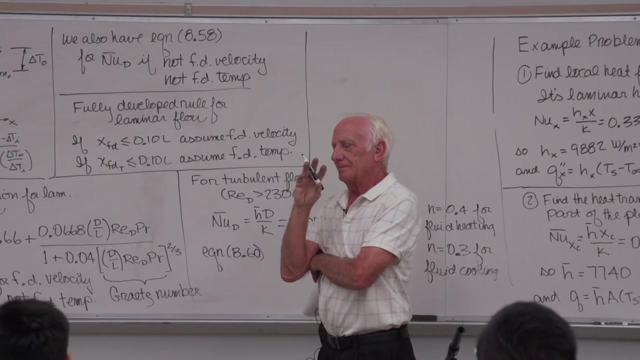 what is it if it's turbulent? You don't ask that question. If it's turbulent? that equation covers both cases. How about fully developed velocity and fully developed temperature? Textbook says reasonably. you just say it doesn't matter. 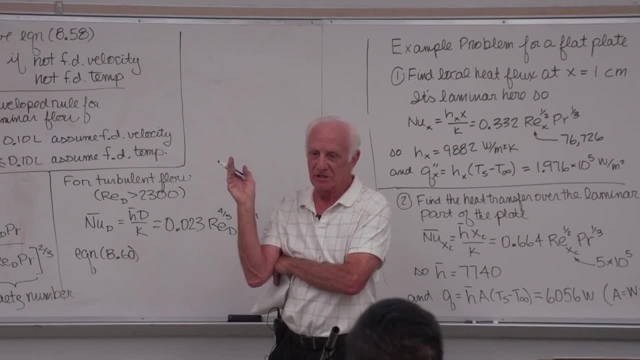 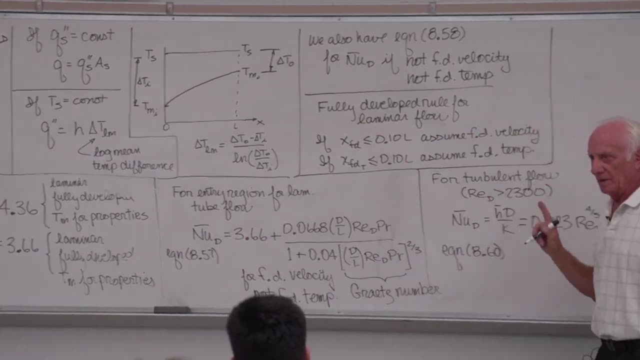 Okay, That one equation works for that. I don't care if it's fully developed or not, I don't care, I don't care, I don't care for turbulent. One equation works for fully developed or not. One equation works for constant tube. 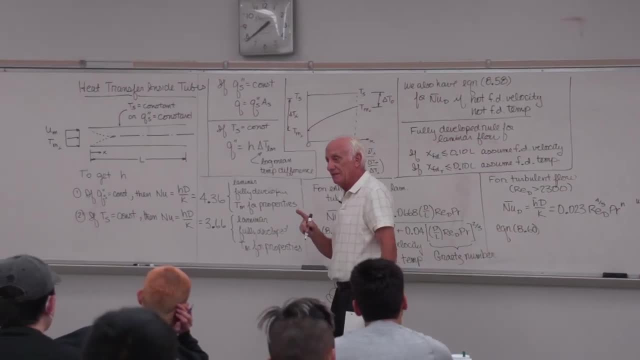 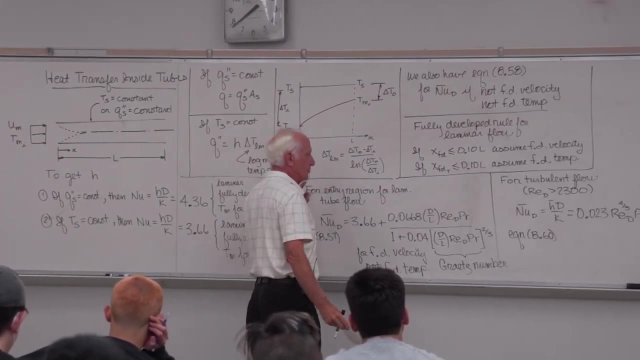 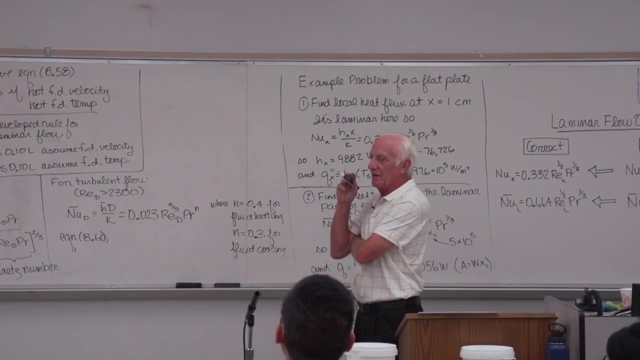 surface temperature or constant tube surface heat flux Makes life easy. How many choices do you have? None, Just one. That's the equation. How about laminar flow? One, two, three, four, four choices to answer. By the way, these tubes are all meant to be smooth. 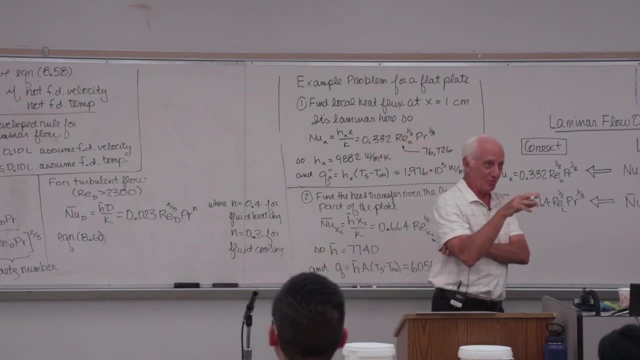 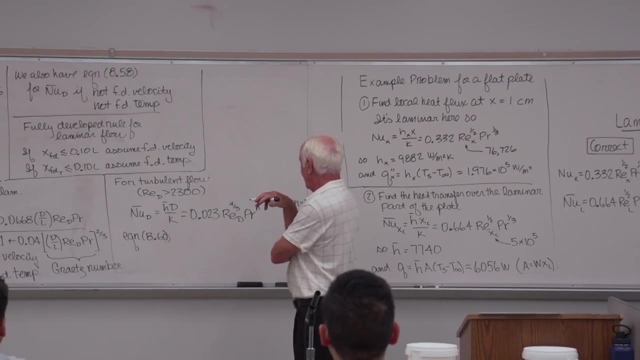 If it's a rough tube, the textbook tells you what to do, But we're looking at smooth tubes, So it's not valid for quote, rough tubes. Okay, So that takes into account any question on this guy. then We're okay, All right. 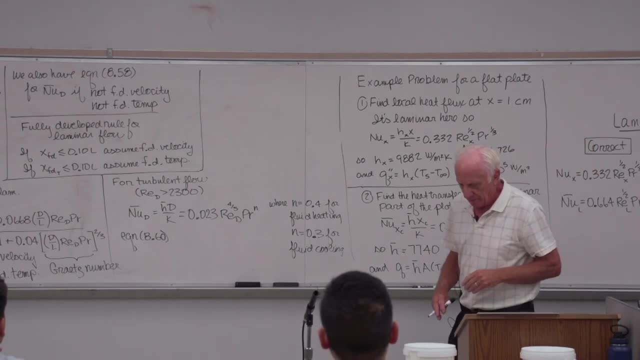 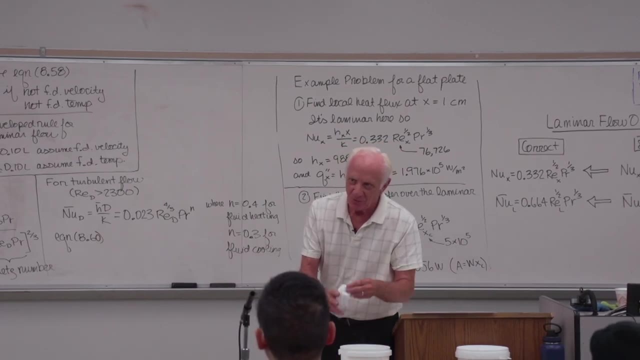 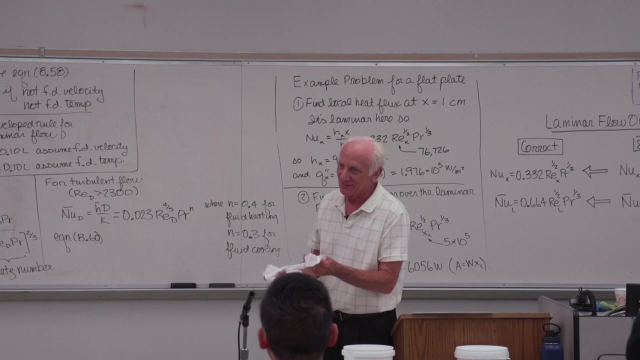 So we're going to work. an example: We have some whiteboard problems, magic wipies. I don't know what happened, but something happened. That's okay. We'll use these guys and paper towels and we'll make it work. 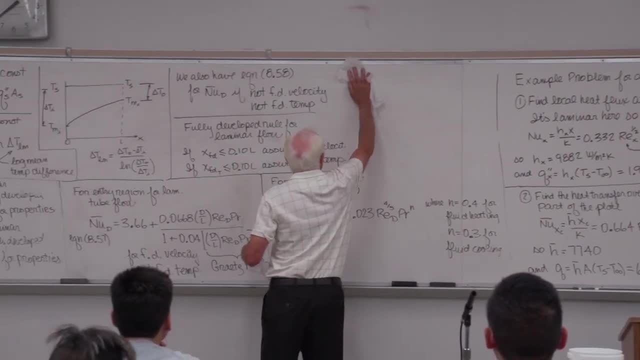 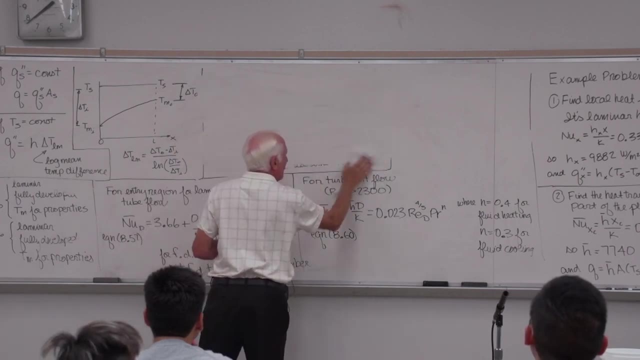 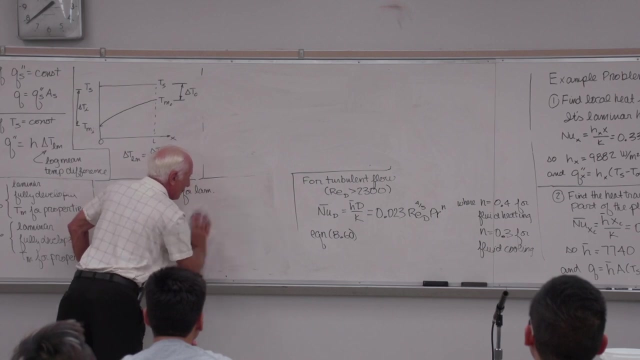 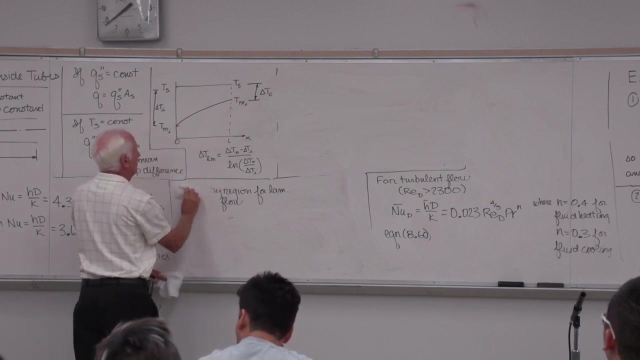 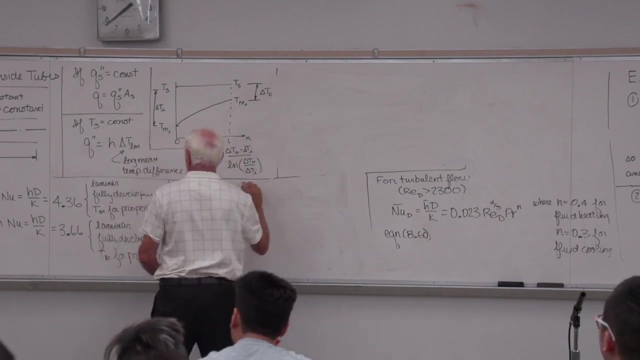 All right. So I'm going to save that guy, This guy I don't want, You don't need him, And we'll just make room. Let's save him. Okay, Save that. Oh, it's okay, I'll get rid of this. 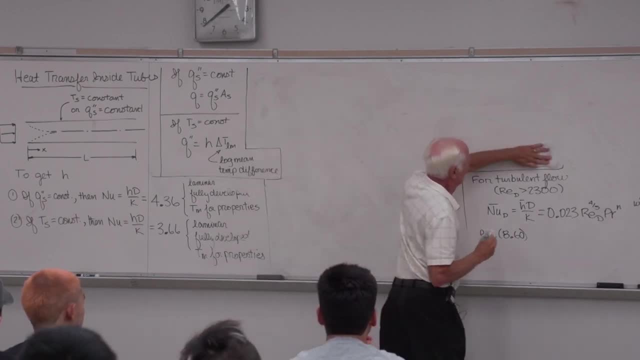 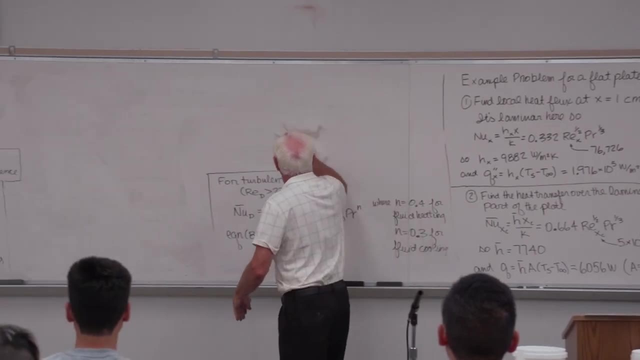 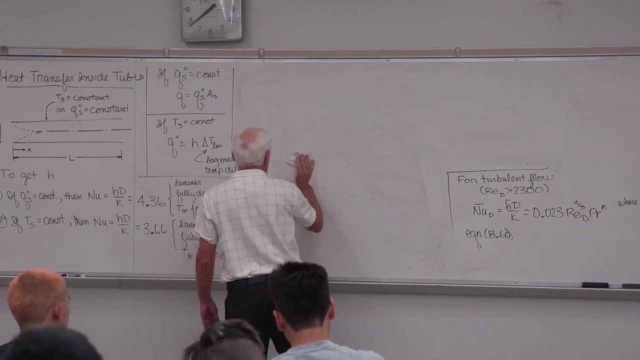 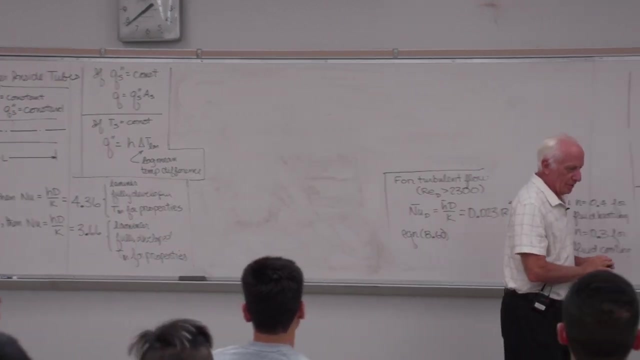 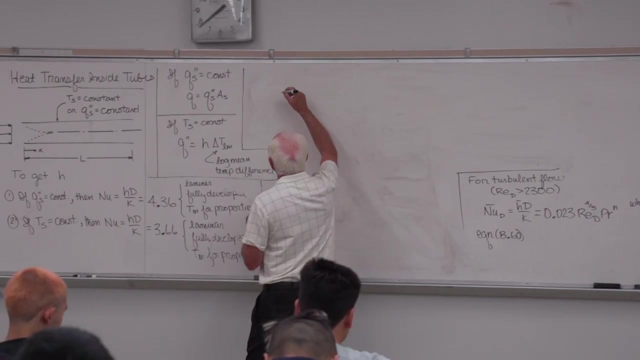 Okay, I think we're pretty good. All right, Let's just make sure it's dry before we put the pen on this. Okay, So here's the problem we have. We're going to be heating water in a tube, So let's see our example. 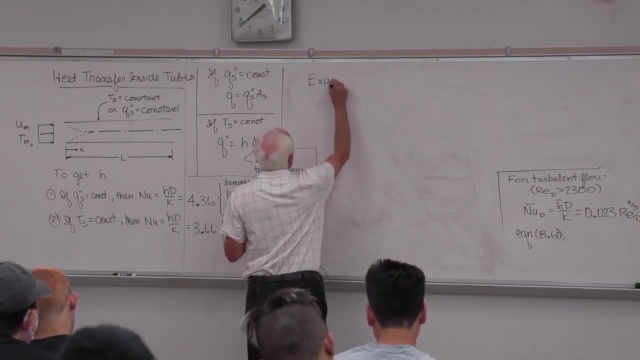 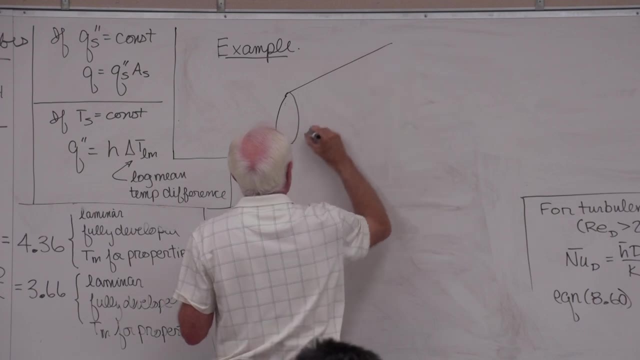 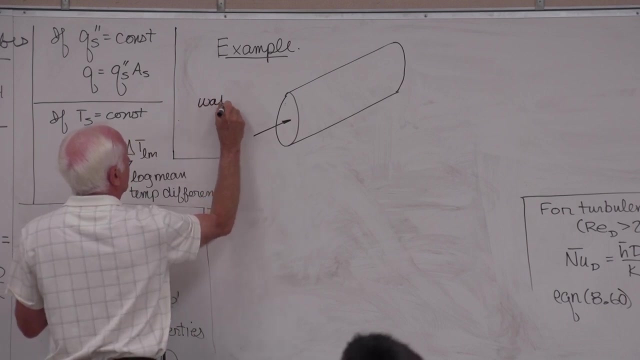 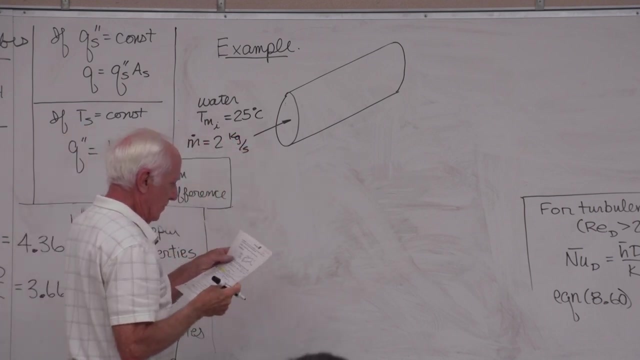 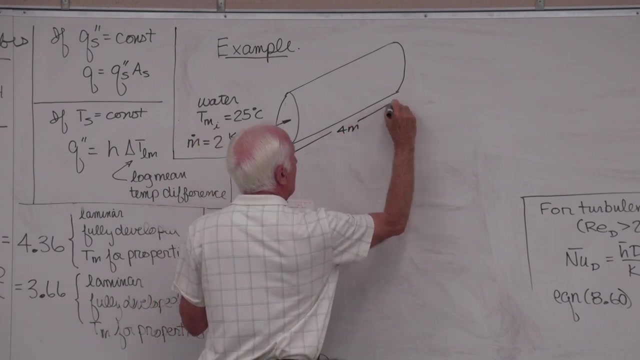 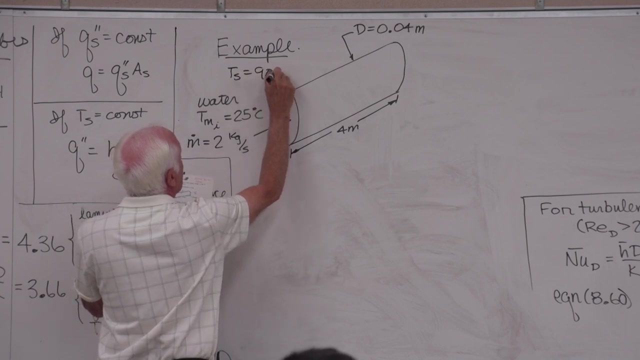 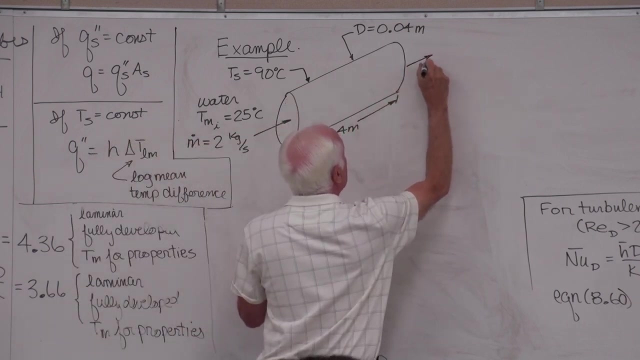 Okay, Water fluid comes in 25 degrees C. mass flow rate: two kilograms per second. Got it Length four meters. Let's see here: Diameter: four centimeters. Tube surface temperature: 90 degrees. Fluid goes out. T mean out. 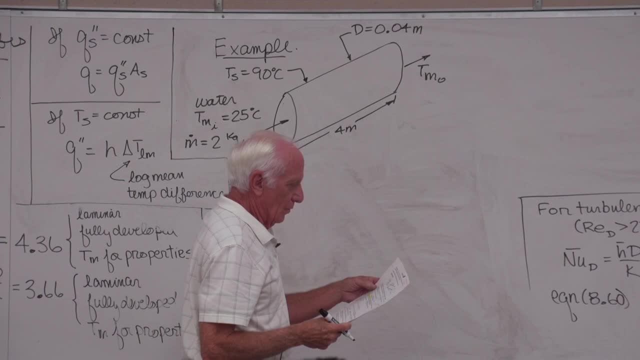 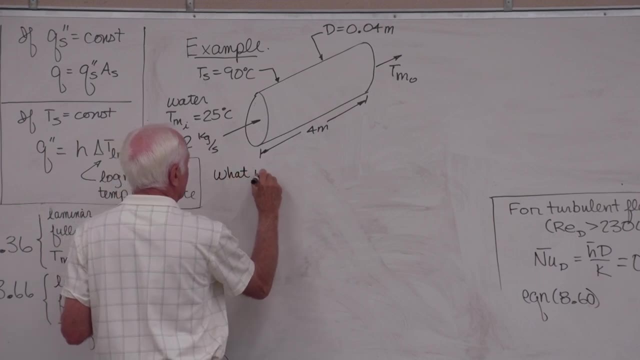 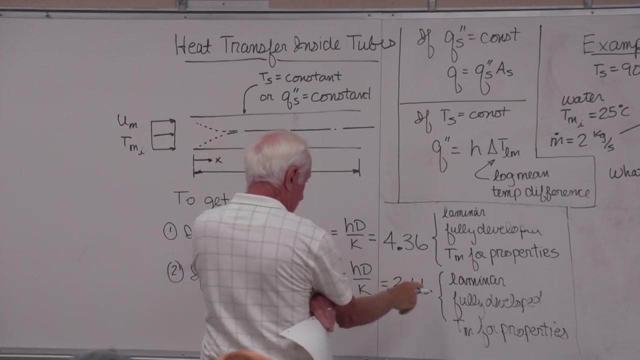 Got it. What is the outlet water temperature and the heat transferred to the water? Okay, We need the Reynolds number, of course. Is it laminar? is it turbulent? We need the Reynolds number. we need the properties, We need the properties. 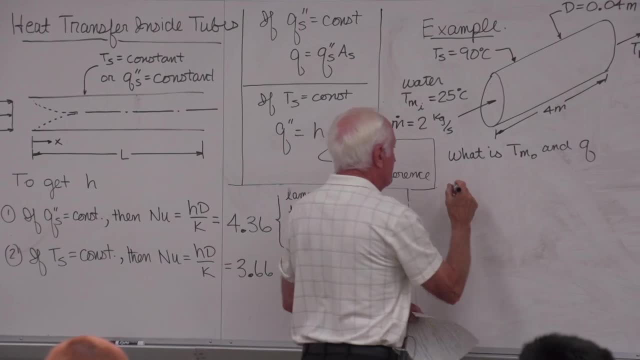 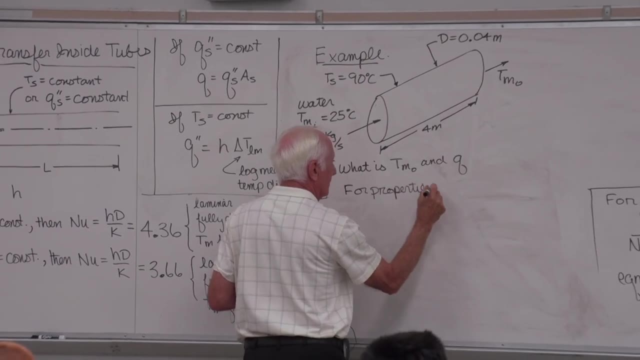 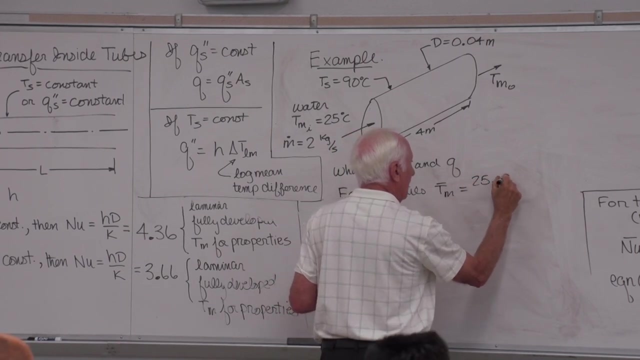 we need the temperature. So for properties T, mean bar equal comes in a 25.. I don't know what it's going to go out at. That was asked for. I don't know what it's going to go out at. I got to guess something. 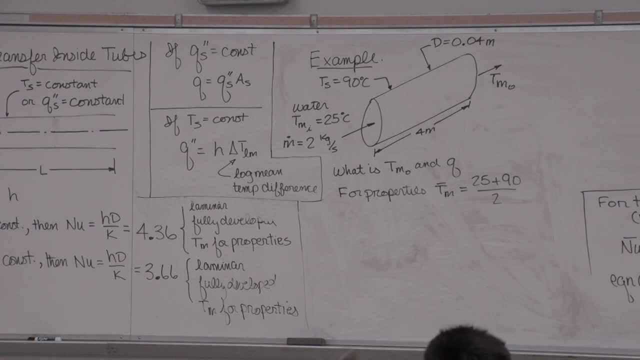 I think you know what. I'll make life easy. I'll guess 25 degrees C. No, it's going to be heated. It's not going out at 25 degrees C. Say, okay, I'm going to guess it. 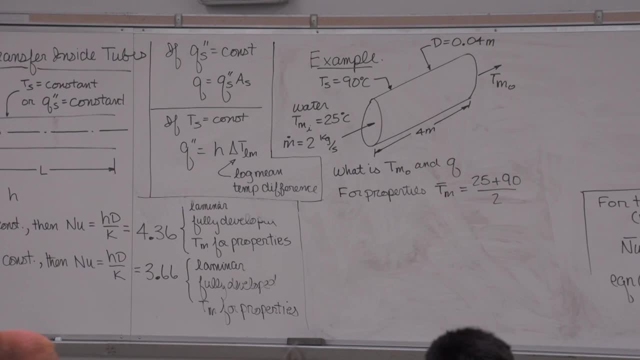 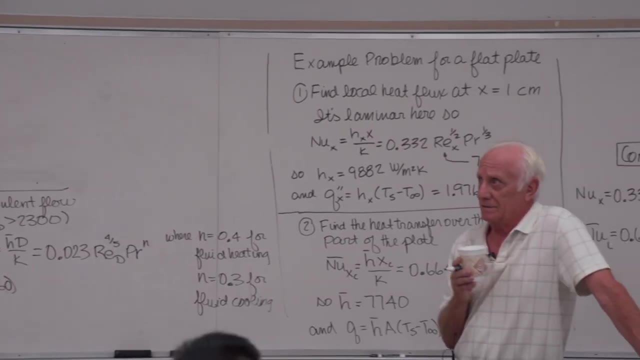 goes out at 50 degrees C. Okay, I can't argue. That's fine, guess, Go ahead and guess it. Most people will say: well, the purpose of that is to heat the fluid as hot as it can get. I'm going to guess it goes out at 90.. 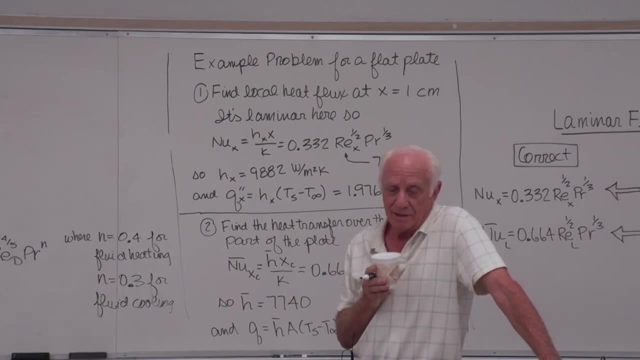 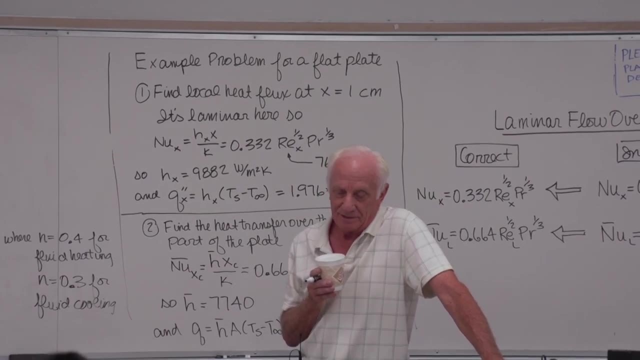 That's a good guess too. I don't care what guess you make, but make a quote. reasonable guess 50, 75,, 90. That's fine. So I guess 90,, just to start. That's a starting point. 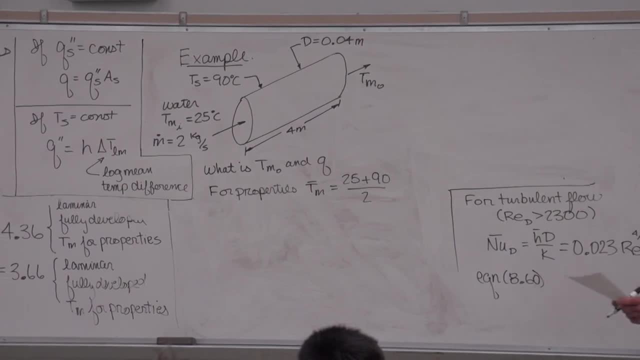 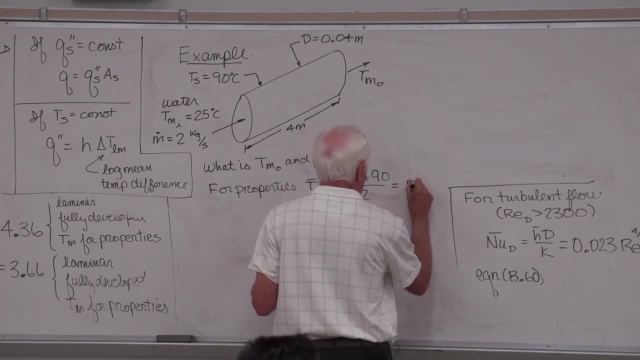 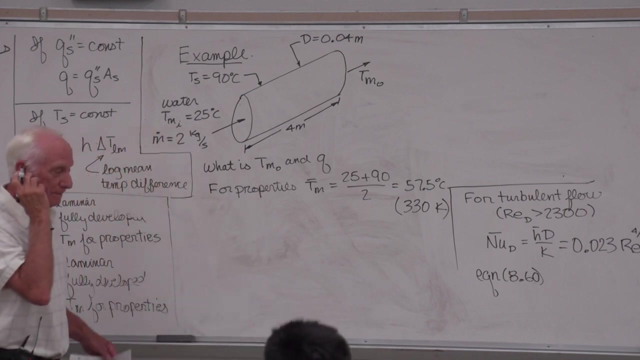 So then, properties of water: 57.5,. but the tables in the back of the book are: in Kelvin, 330.5,. I just say 330.. Go to the back of the book, get the properties. Okay, got it. Then get the Reynolds number. 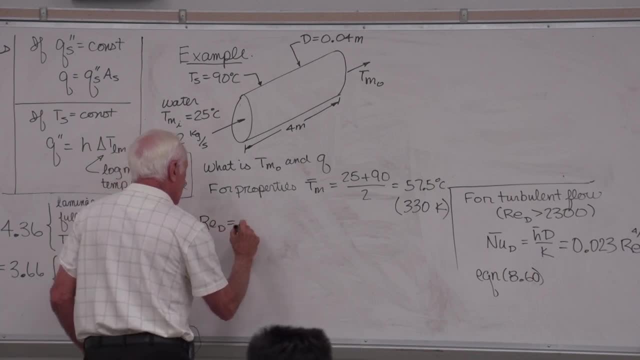 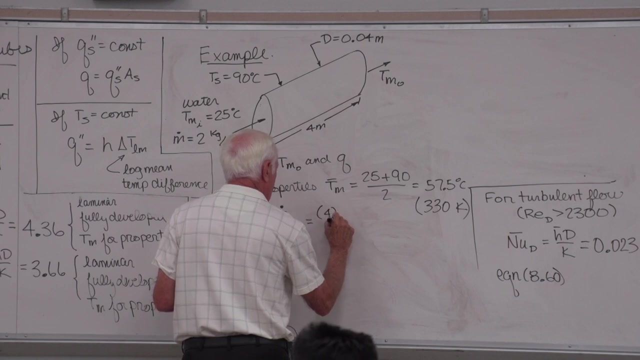 Reynolds number based on diameter. Okay, So don't use velocity. I told you last time We're using mass flow rate. 4M dot over pi. Demu d is four centimeters. Yeah, Back of the book. kinematic viscosity: 528 times ten to the minus eight. 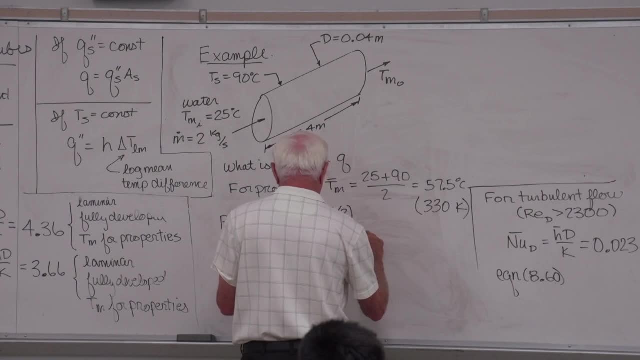 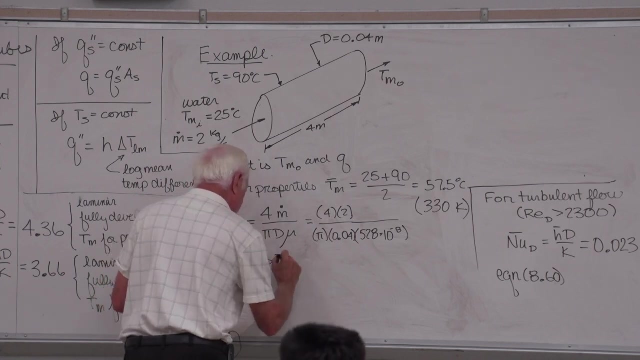 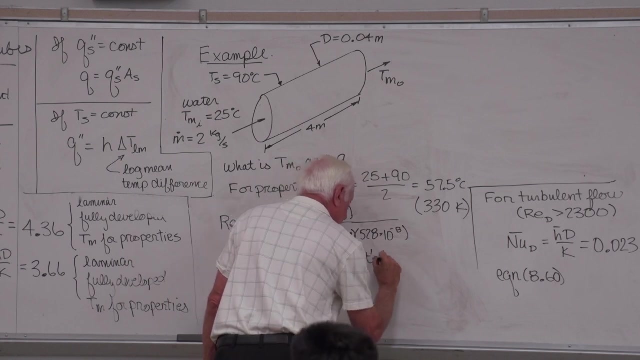 I think that is Reynolds number based on diameter: 121 times 10 to the fifth. It's way greater than the magic Reynolds number 2,300.. So yeah, it's turbulent flow. Got it There. he is right there. Turbulent flow. There it is. 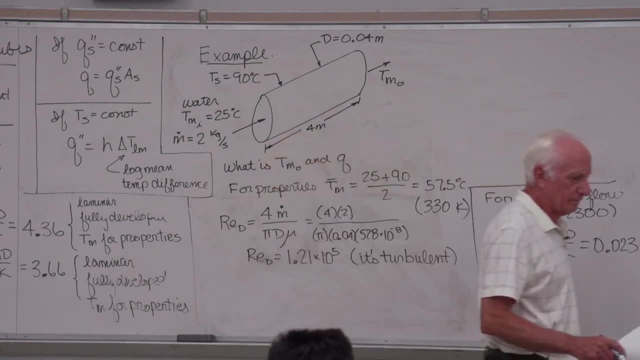 Use equation 860.. Okay, Is the fluid being heated? Of course it is Fluid being heated- 0.4.. So we go ahead and we use 0.4.. Let's see if we can get that thing cleaned up there. 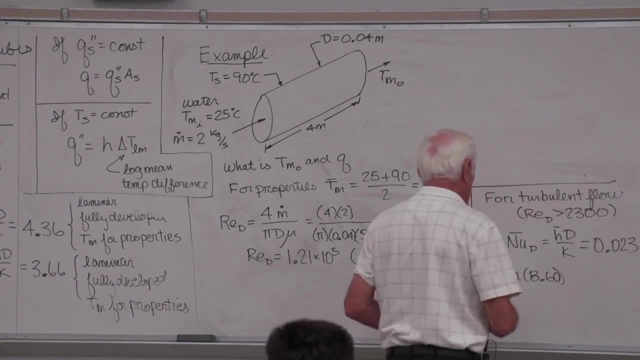 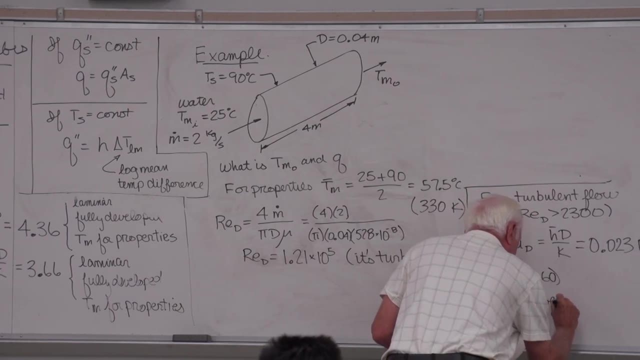 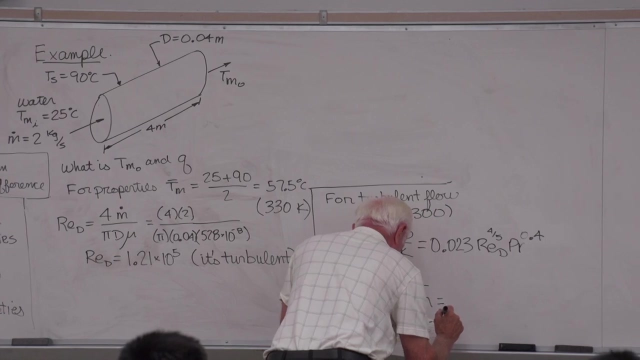 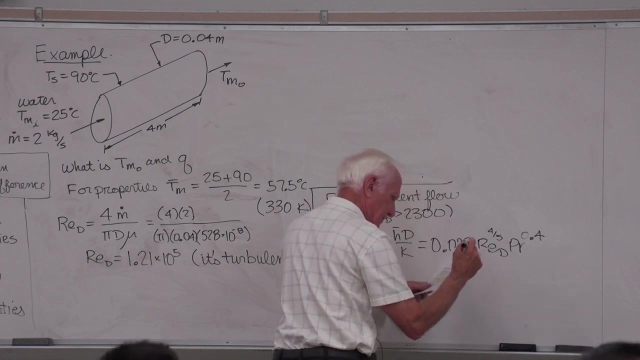 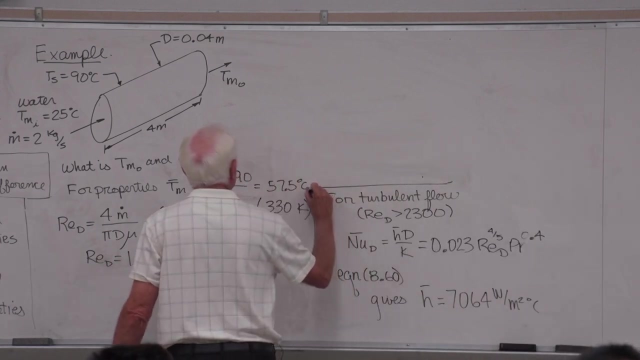 Okay, Equation 860, put everything in there and this gives h-bar 7084.. Okay, Make sure that's right: 7064.. Okay, So we've got that Now. second thing: let's go upstairs with that h. 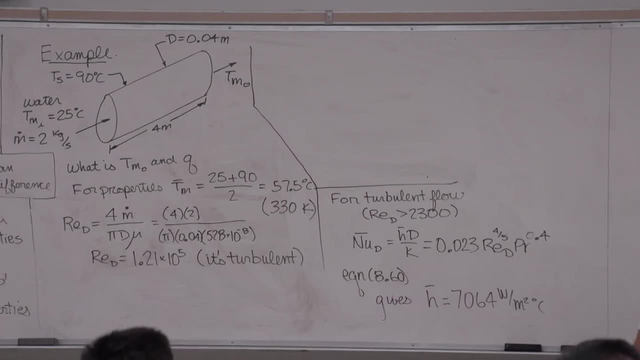 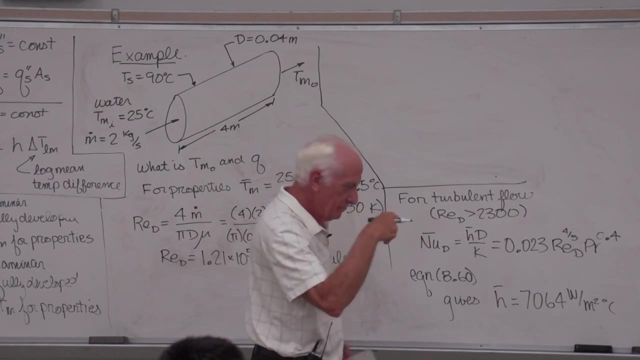 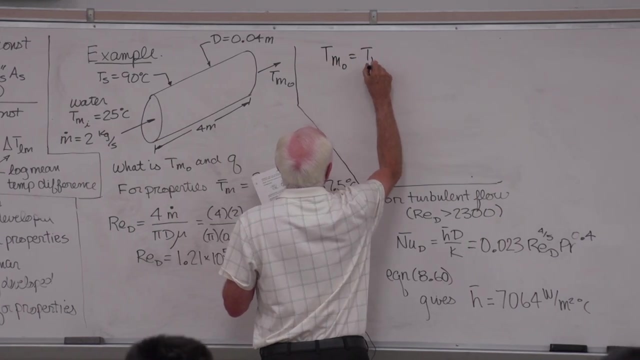 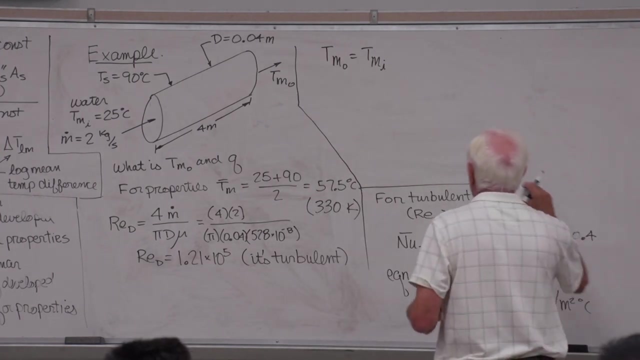 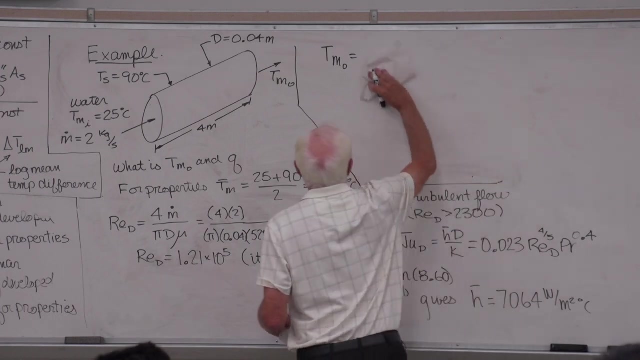 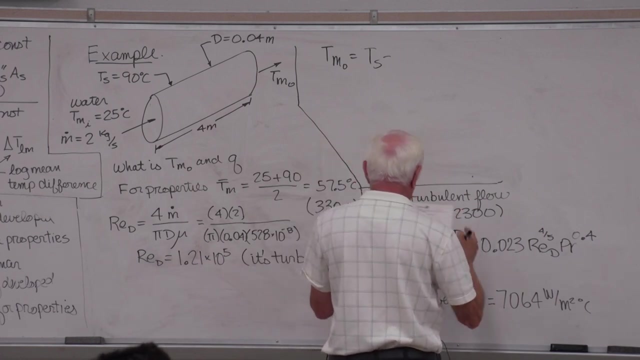 and now we have to find T mean out. Okay, In your notes from last time, here's the equation for T mean out T surface. that should be: T surface minus T. surface minus T mean in. Okay, T surface minus T. surface minus T mean in. 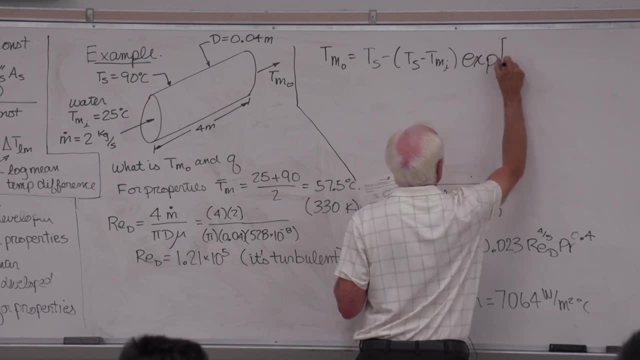 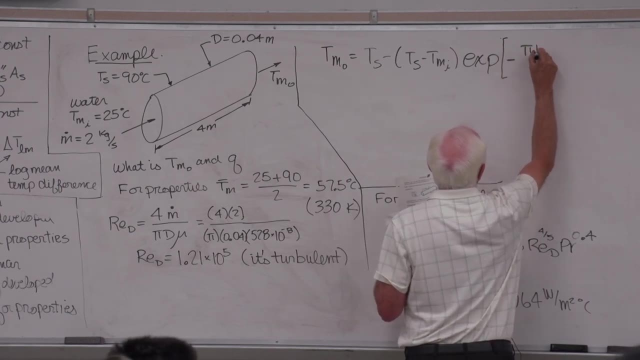 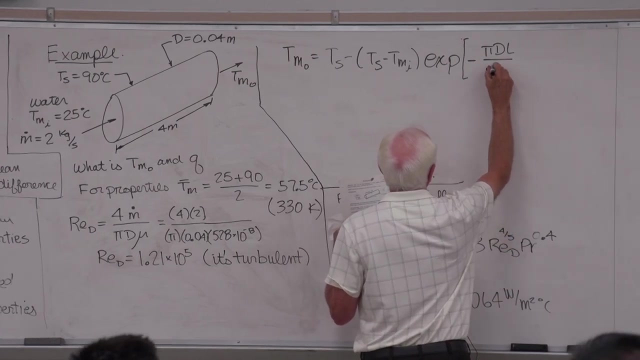 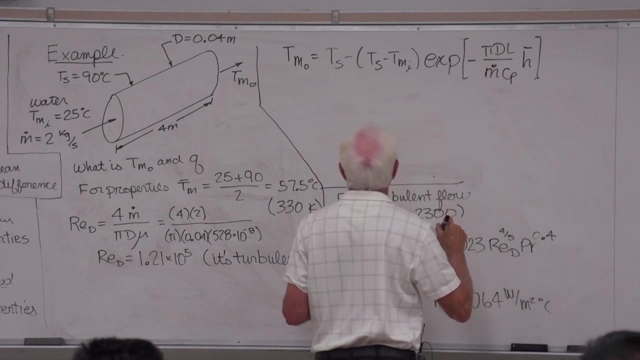 Times. exp exponential minus Pi dL divided by m dot: cp times h-bar, Times h-bar, Times h-bar. I know it all. I know Ts. I know T mean n. I know Pi D L, M dot, I know. 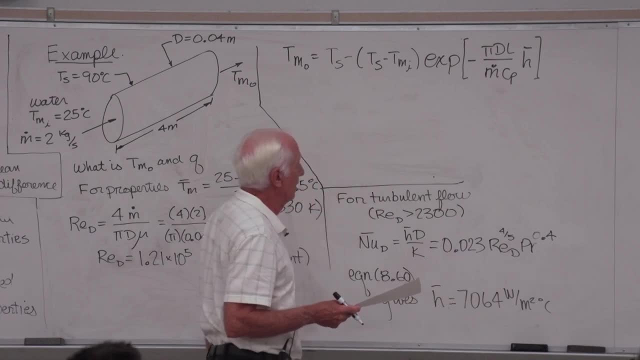 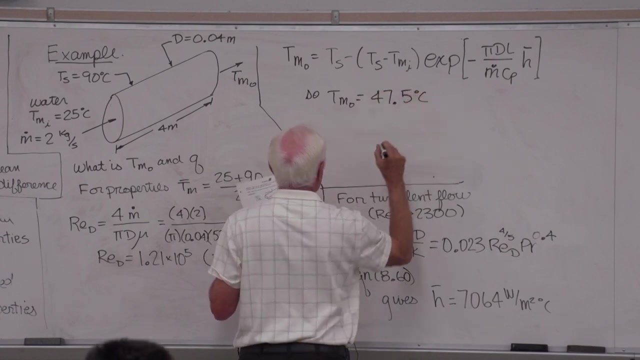 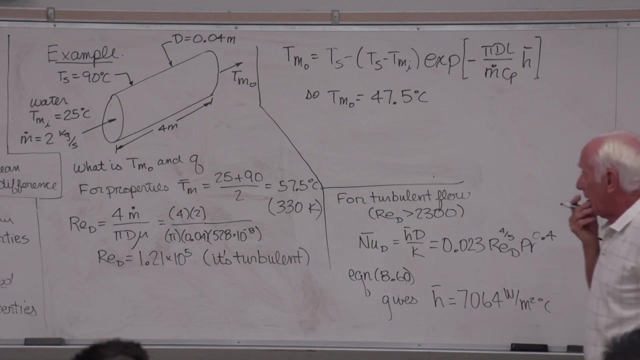 C is a P. I know I just found H bar 7064.. Put it all in there. So T mean L, 47.5 degrees. C Got it. Now I got to find Q. Let's do the easy way first. 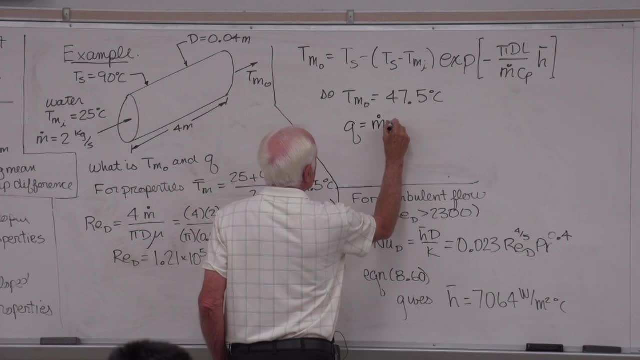 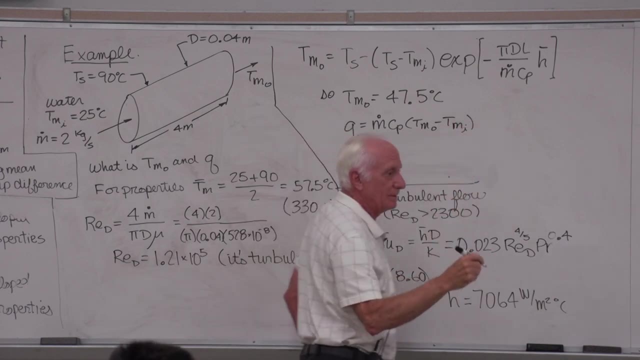 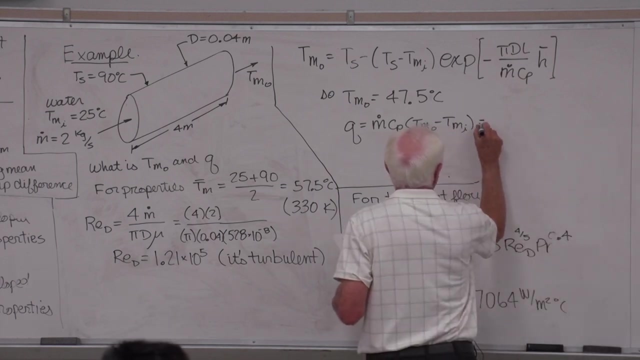 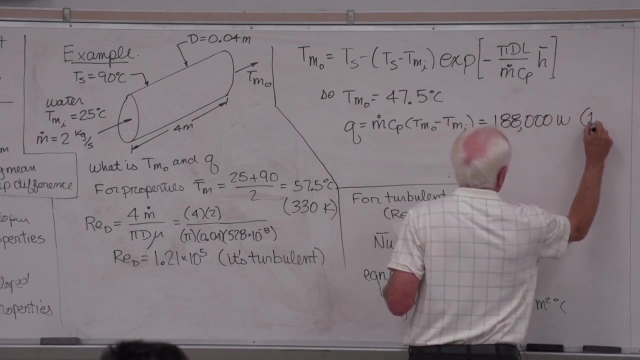 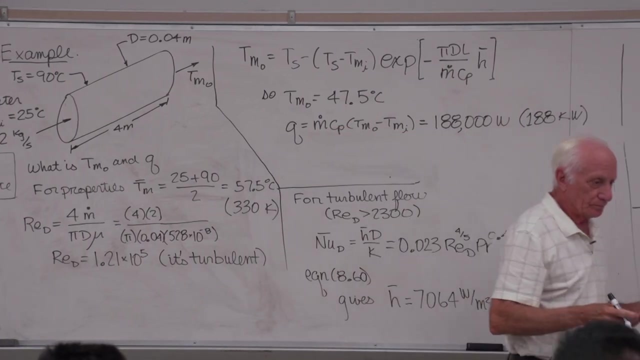 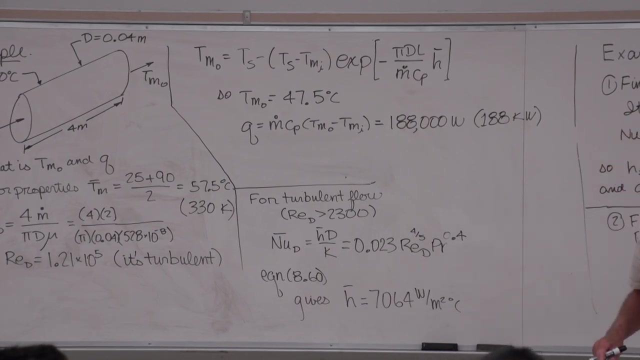 Q equal M dot C sub P. T mean mean out, minus T mean in. I just found T mean out, That's the easy one: 188,000.. 188 kilowatts. So I found Q. All right, Let's take a look at. I need space. 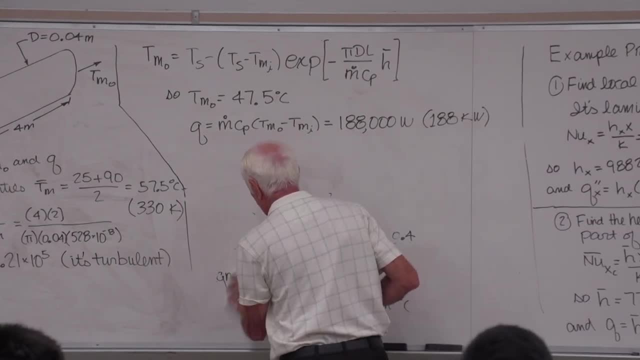 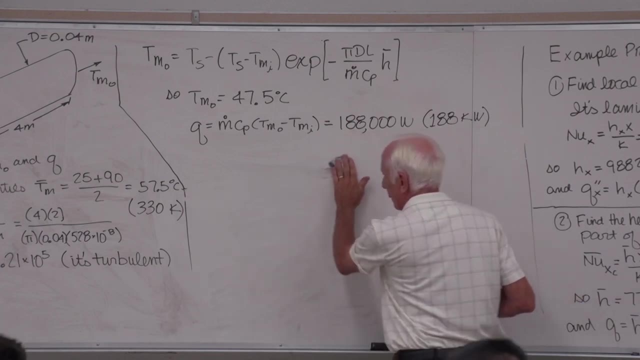 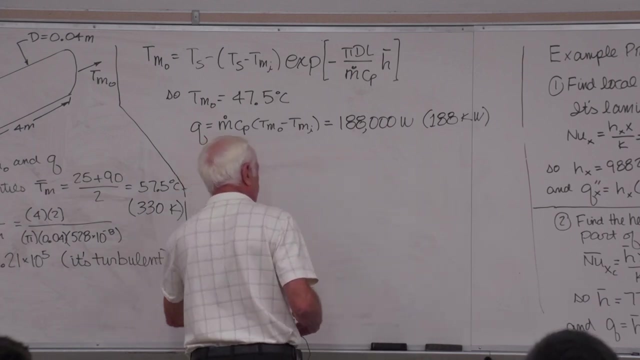 so I'm going to get rid of this stuff. If you don't want to do it that way, you can do the log. mean temperature difference. 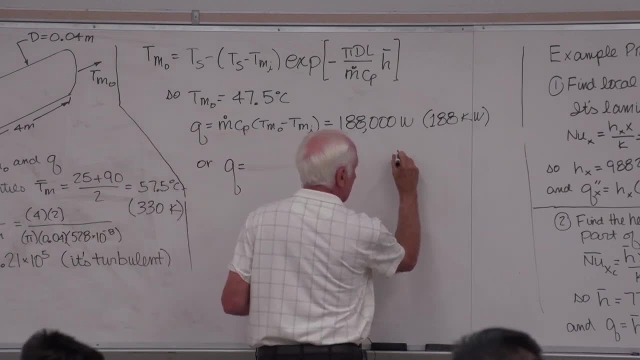 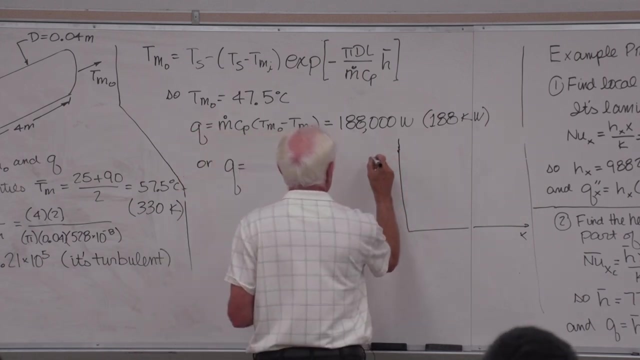 Let's make a plot of this guy. Come and see, it's okay. This is constant tube surface temperature and that tube surface temperature is 90,. so 90 degrees here. The tube length is four meters, comes in at 25,. 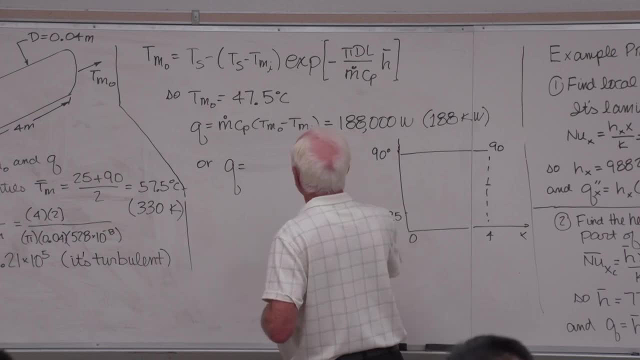 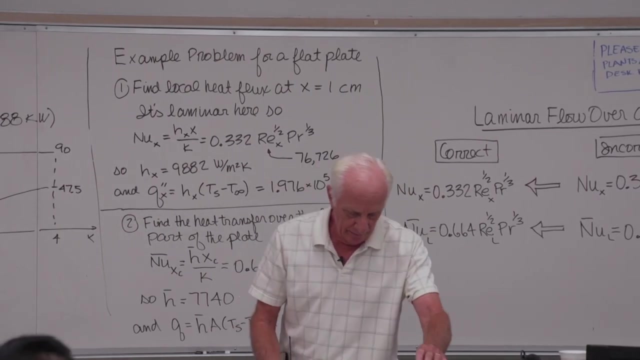 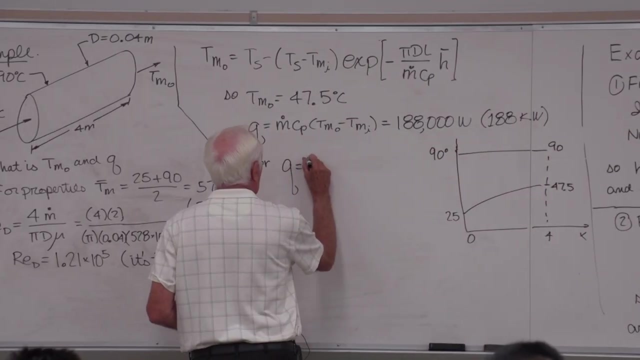 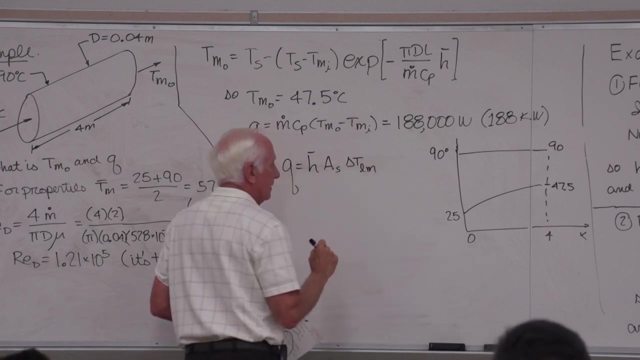 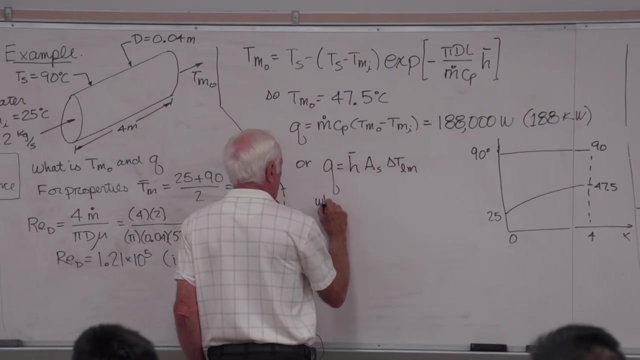 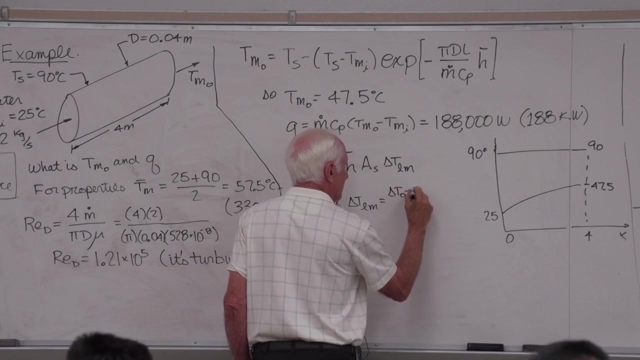 it goes out at 47.5.. So that's how the temperature looks as it goes through there. Then we'll put the area in. So Q equal h bar surface area. Delta T log mean. where Delta T log mean equal Delta T out minus Delta T in. 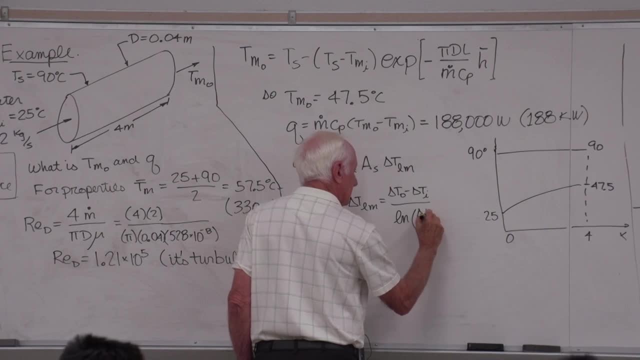 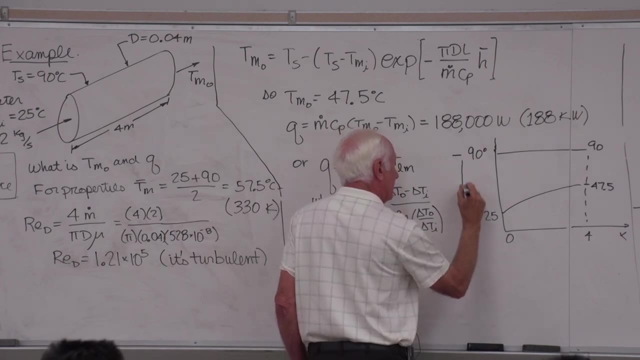 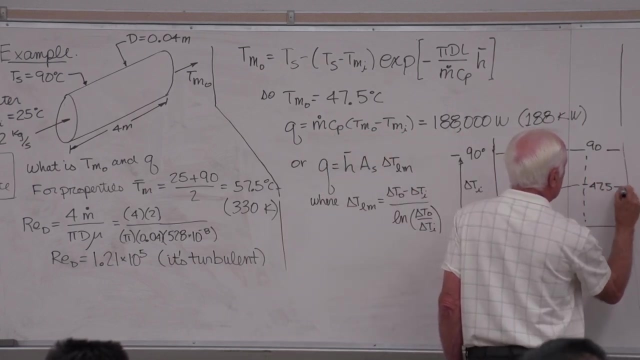 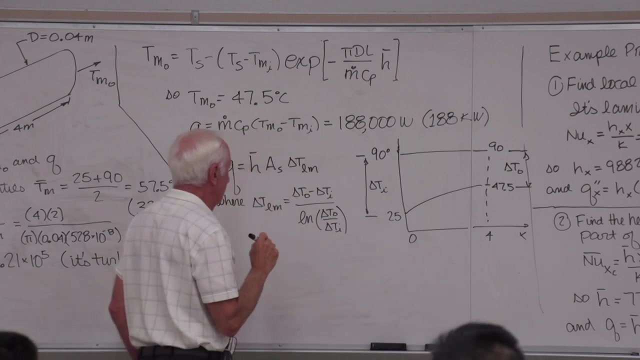 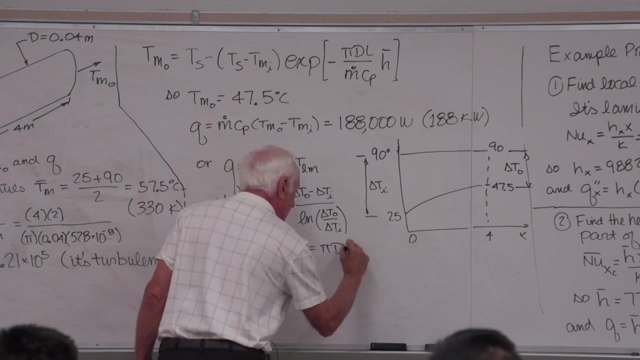 divided by the natural log: Delta T out minus Delta T in. Here's Delta T in, 90 minus 25.. Here's Delta T out 90 minus 47.5.. The surface area of a tube: Pi D L, circumference times length. 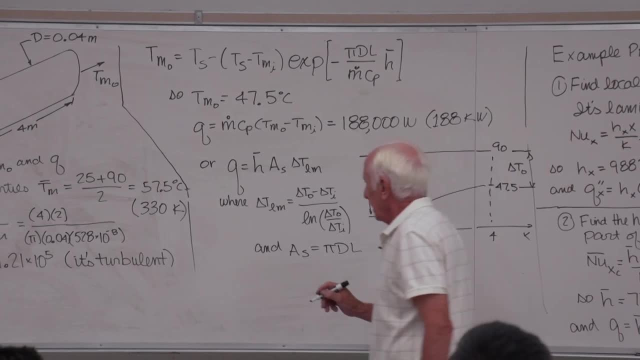 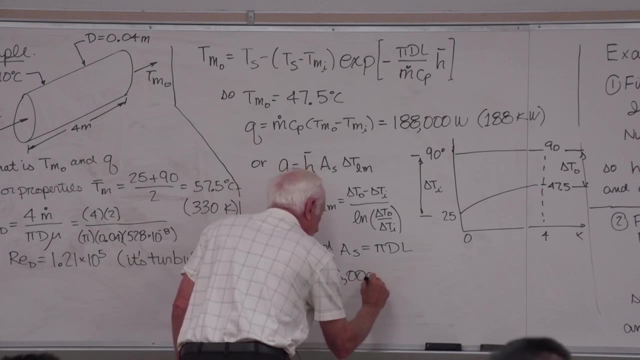 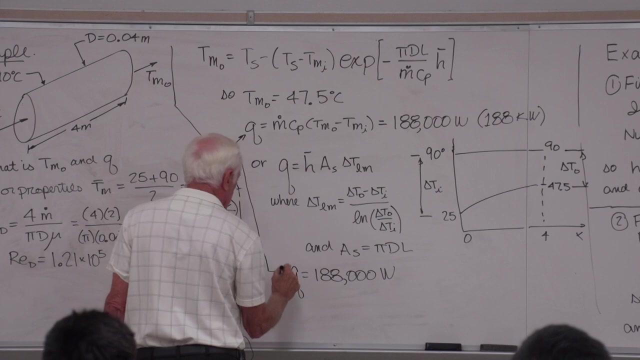 put that in there. If you do that, Q equal 288,000 watts. Of course, same answer. You can do it either by m dot C sub Pt or you can do it by the log mean temperature difference. Generally it's easier than m dot C sub Pt. 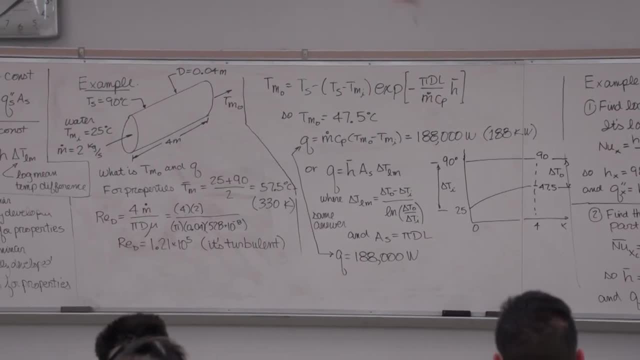 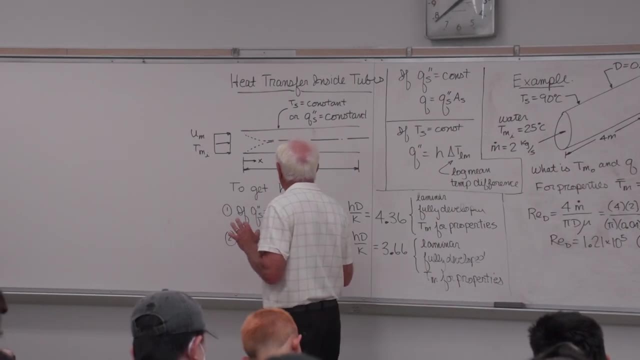 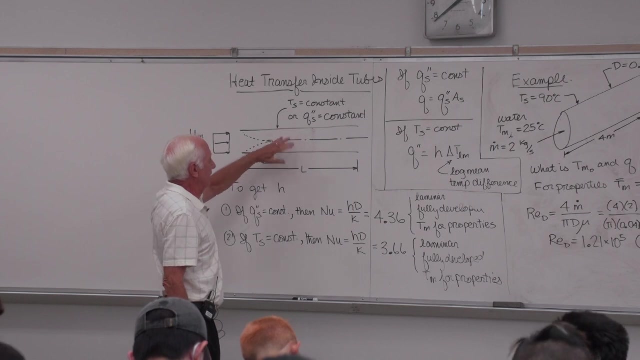 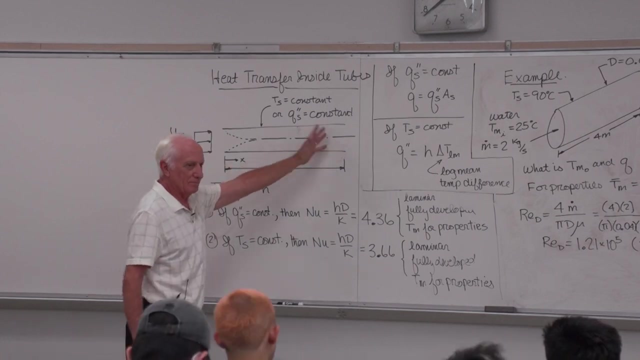 Pt equals P, T power equals Pt. But sometimes that's not an option. For instance, what if the problem said: I'm gonna put 188,000 watts into that fluid? I wanna do that, So the temperature comes off to be blah, blah, blah. 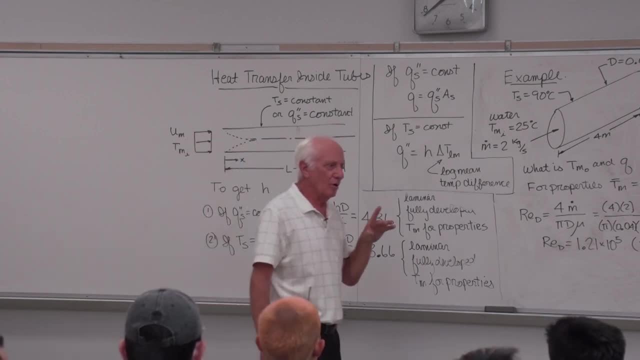 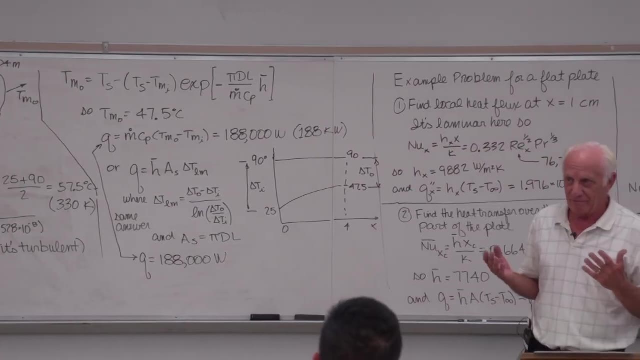 How long should the tube be? Here's the question: How long should the tube be? tube B: Well, what do you do? Well, you get out your library of equations for tubes and you try and find somewhere the symbol L. You hope. 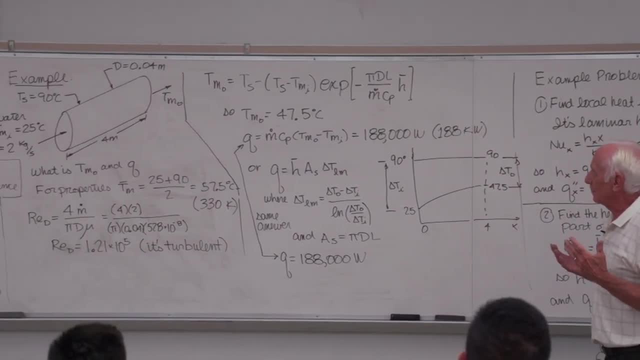 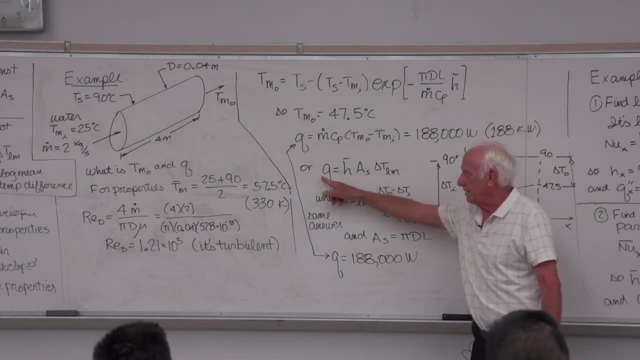 you find L in the equation somewhere. Let's see where is L. There it is right there. There it is, He goes up there, right there. Yeah, if I know Q 188,000 and I can find T mean out. 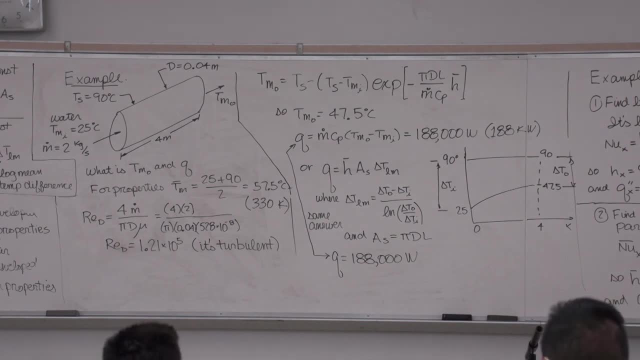 I can solve for L. That's when you would use that equation. as opposed to M dot C sub PT, There's no L in M dot C sub PT. Of course these answers aren't right at all. They're not right. Now I know that. 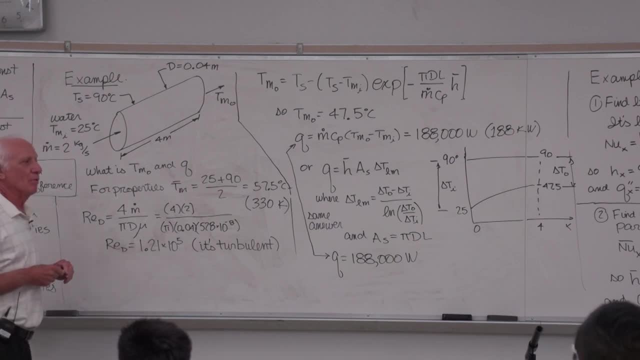 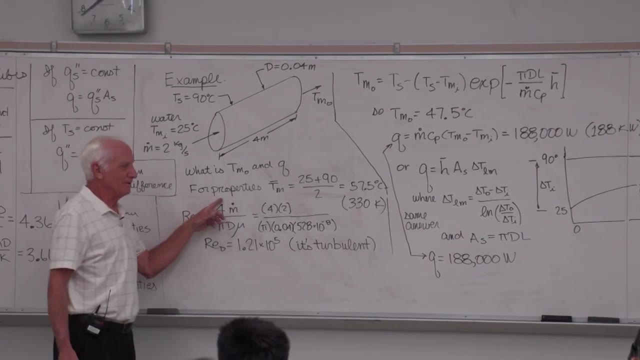 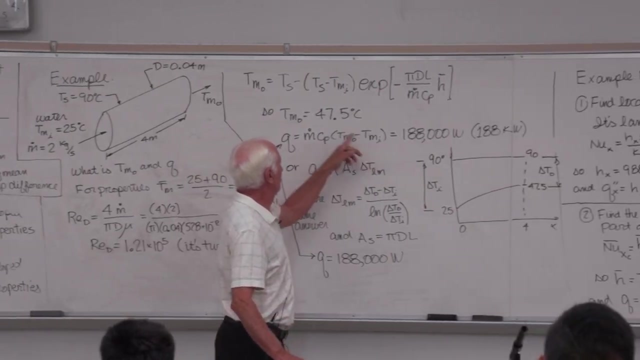 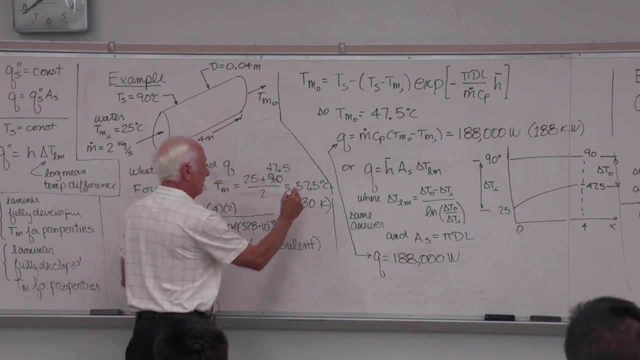 Why aren't they right? Go way, way back to the first line that you started with For properties. did it come out at 90?? No, not even close. Not even close. Closer to 50, 47.5.. Get a new temperature. 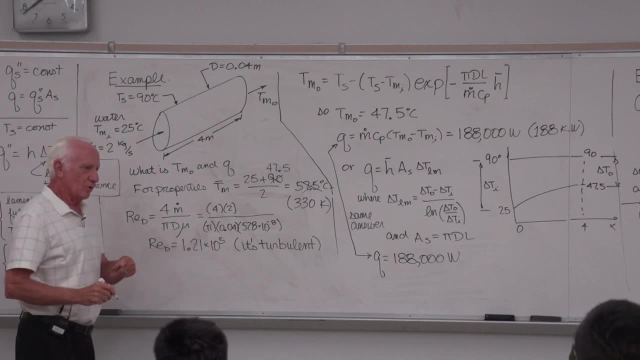 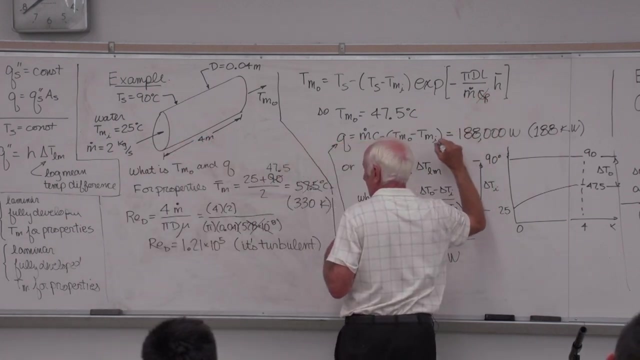 It won't be that. Go to the back of the book. Get the properties at that temperature Mu changes. Is it still turbulent? I hope so. Does C sub P change? Yes, Is T mean out going to change? Of course, 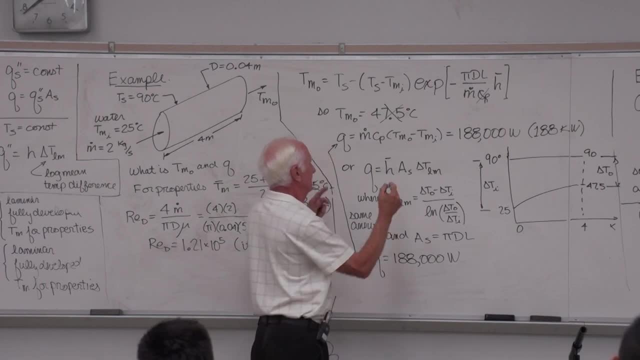 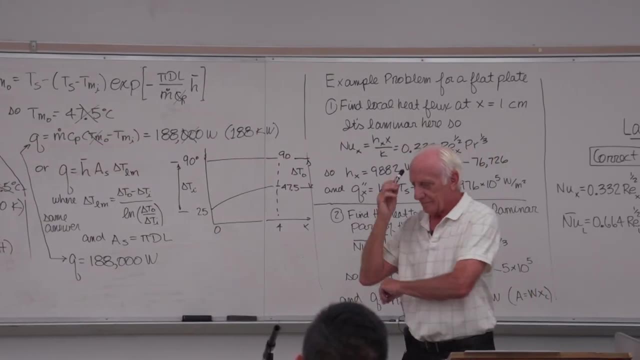 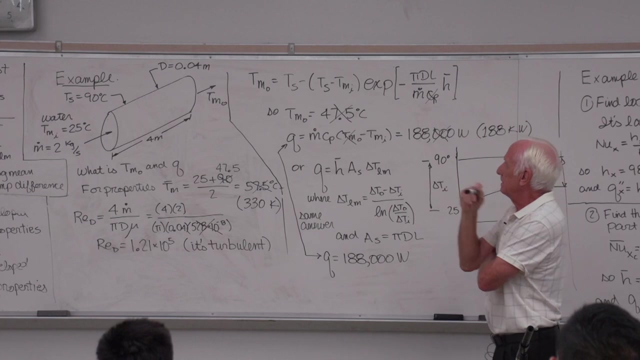 T mean out changes. Does Q change? Of course, Yeah, So you go through it another time. and now the temperature stopped to be maybe 48.7.. You say I'm within a degree, almost there, But you know what I'm going to try and get to: within a half a degree. 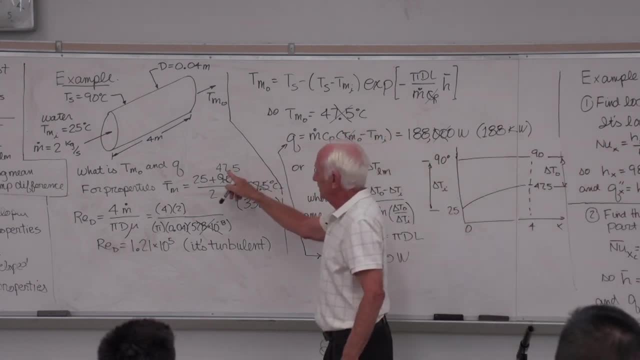 you do it one more time, Get a new T mean out, Put the two T mean out here, Go through the whole procedure one more time, and now you get 47.8.. And the last time it was 47.7.. Oh, I'm within one tenth degree C. I'm going to stop. Close enough, I'm done. So the point: 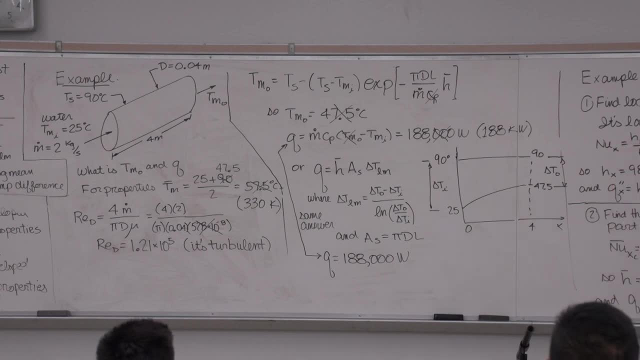 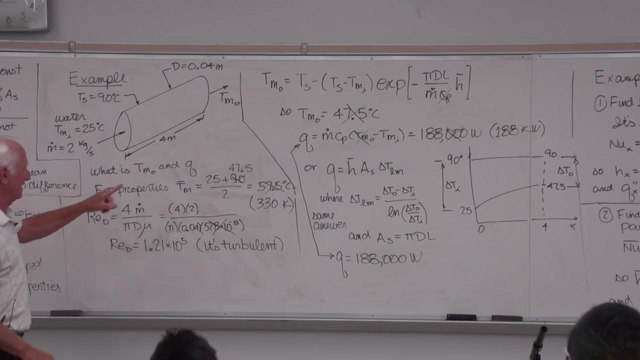 is you iterate until you converge at what you think is reasonable to converge to. But in the textbook and in the class here and on the midterms and the final you don't do that. You go through it one time. You make what you think is a reasonable guess for that. 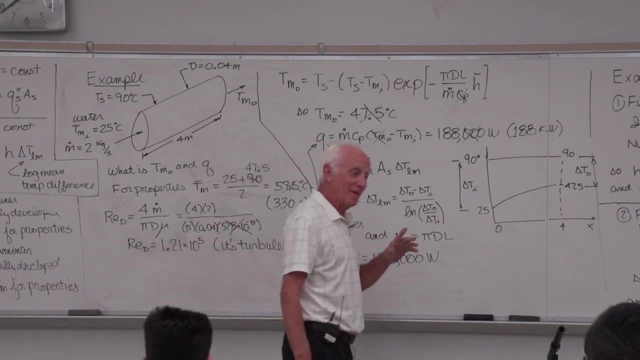 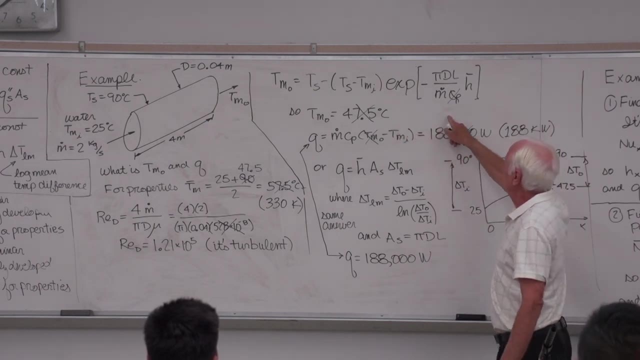 temperature here. And then you go through it one time and say I would repeat the above. When you're all done right here, you say I would repeat the above. calculations with a new T mean for properties. But don't do any more work, But tell me what your next. 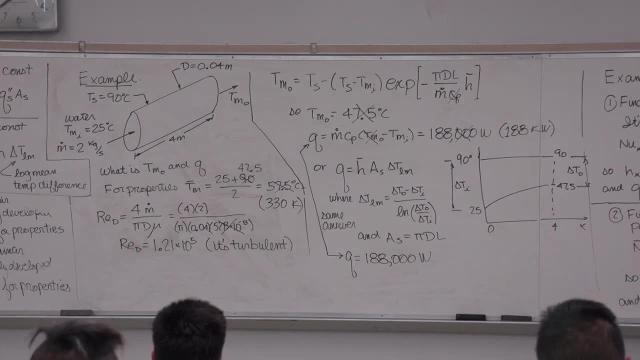 guess would be for an iterative procedure. Now, this was the easiest way to do it. This is the easy problem, This is the turbulent problem. On Friday we're going to work the much more difficult one, the laminar problem. So I think we'll stop for today, And so Friday.